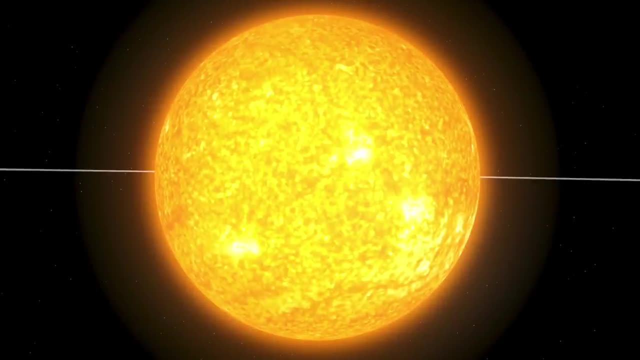 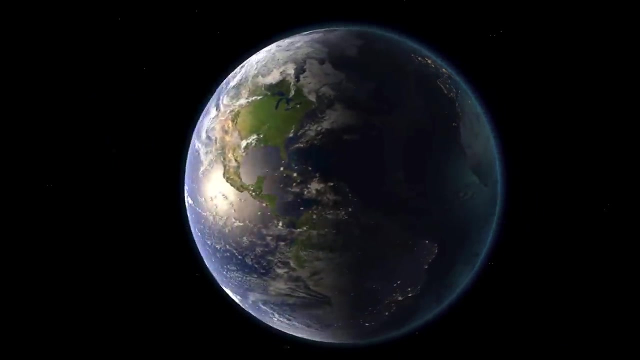 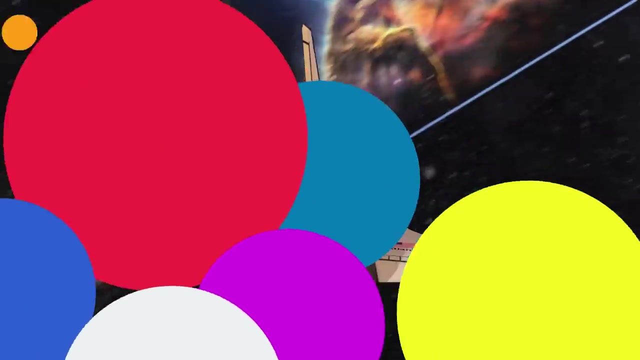 and the star that's closest to us is called the Sun. We live on one of the rocky planets and we call that planet Earth. Do you know where on planet Earth you live? Hey, that's where Lizzy lives. Alright, this is going to be fun. 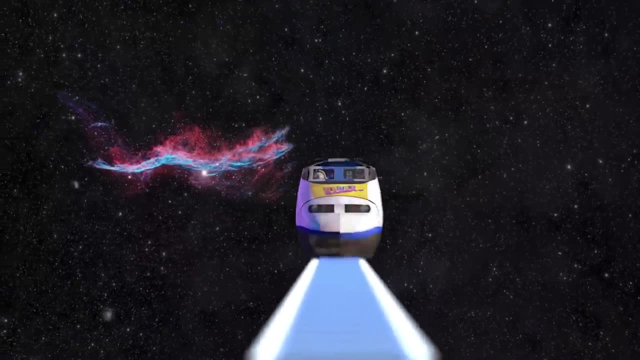 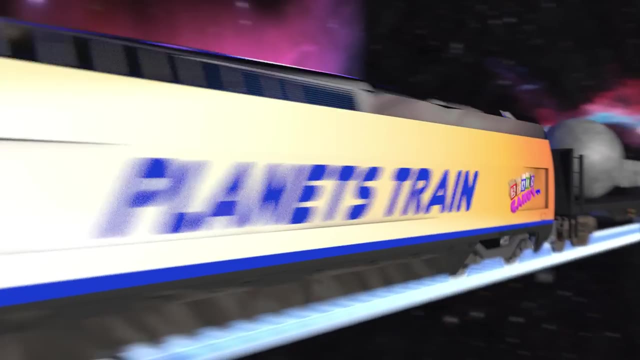 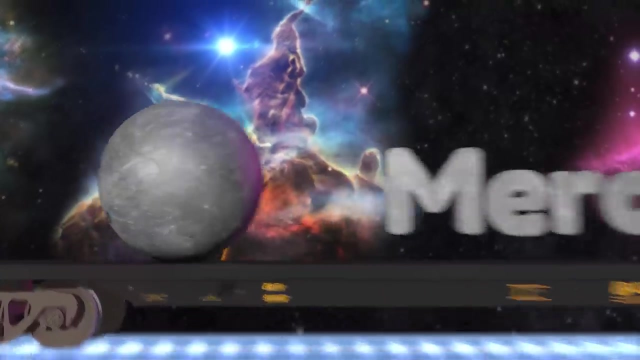 Here comes a big space train with models of all the planets in our solar system. Let's join Lizzy on the planet's train to learn a bit about each planet. The closest planet to the Sun is Mercury. It's very small and mostly made of rock. 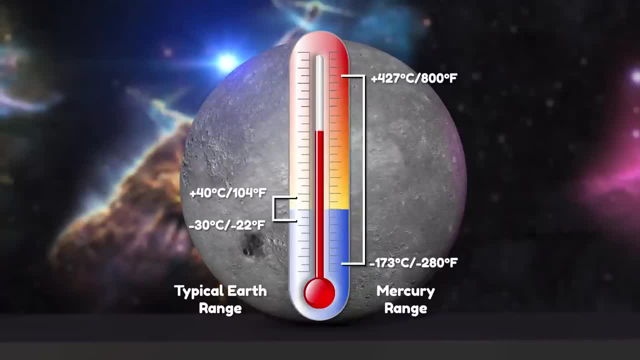 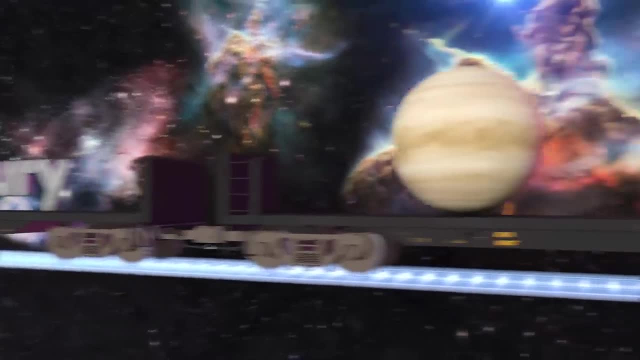 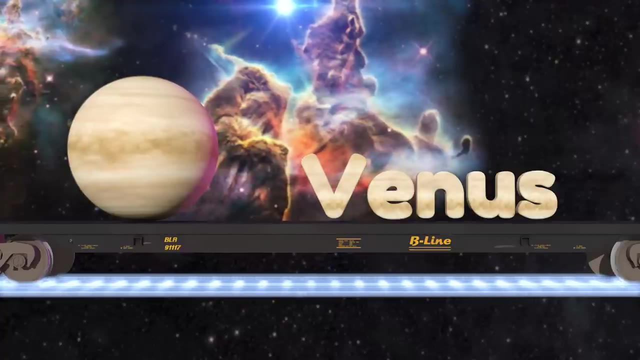 Daytime on Mercury is really hot, but the nights are super cold, giving Mercury the biggest temperature range of all the planets. The second planet from the Sun is Venus. Unlike Mercury, it's covered in a thick layer of clouds and it's the hottest planet in our solar system. 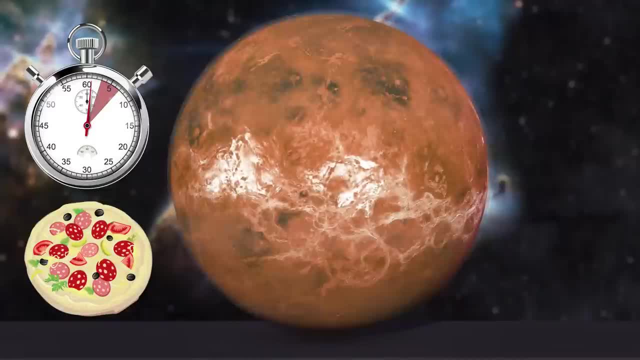 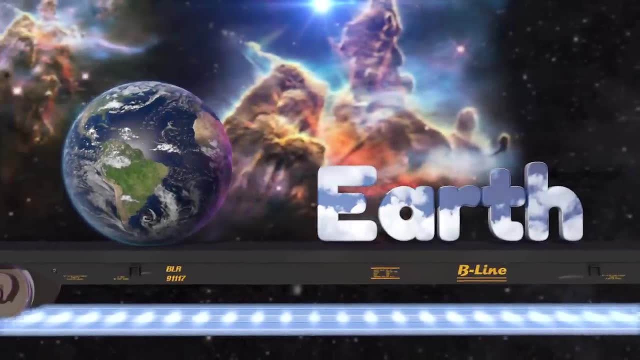 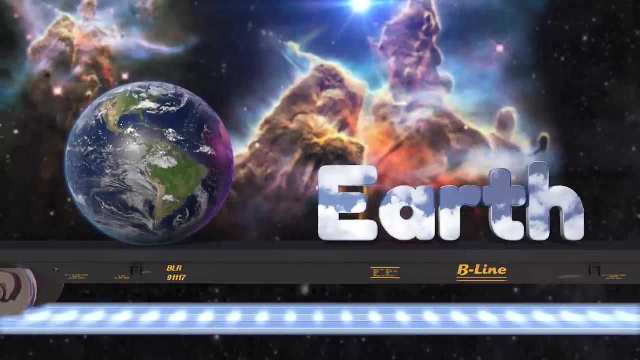 The surface of Venus is so hot that it could cook a whole pizza in only three to seven seconds. The third planet from the Sun is called Earth, the one we all live on. It's the only planet we know of that contains life, but scientists are constantly looking. 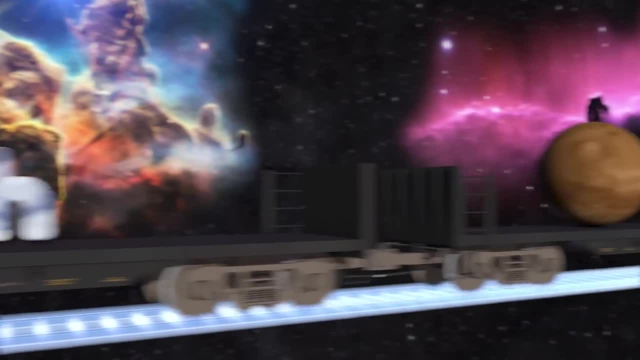 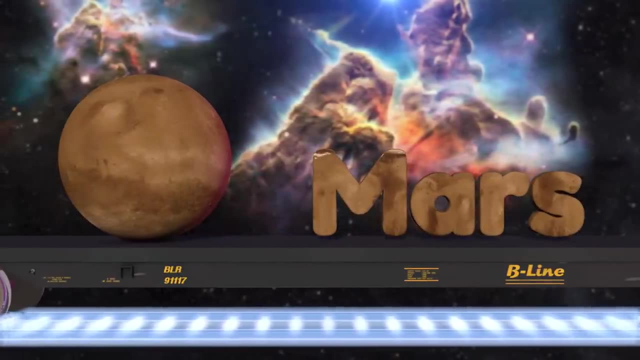 for signs of life on other planets. The next planet is Mars. It's covered in rocks and dust and is about half the size of planet Earth. We hope to send people to Mars by the year 2035, or maybe even sooner. 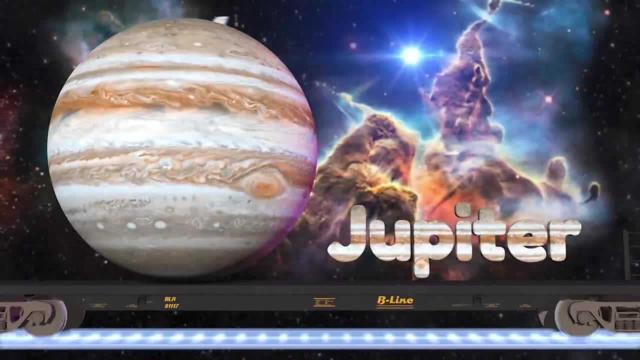 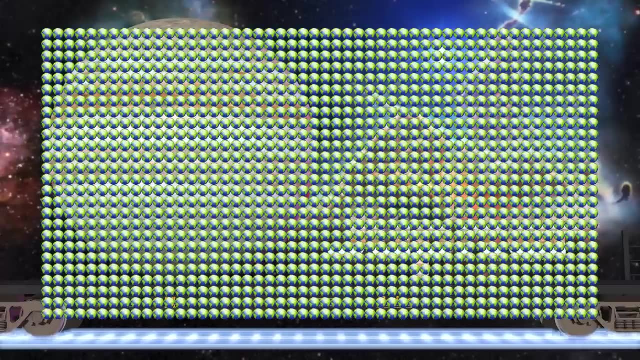 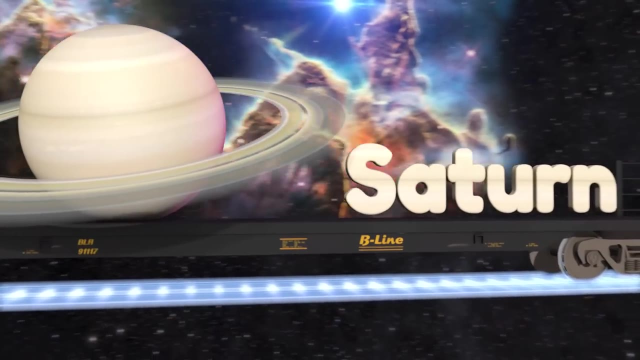 Next up is the gas giant Jupiter. It's the biggest planet in our solar system and it's so big you could fit around 1300 Earths inside of it. Saturn is the second largest gas giant planet and it has a beautiful ring system around it. 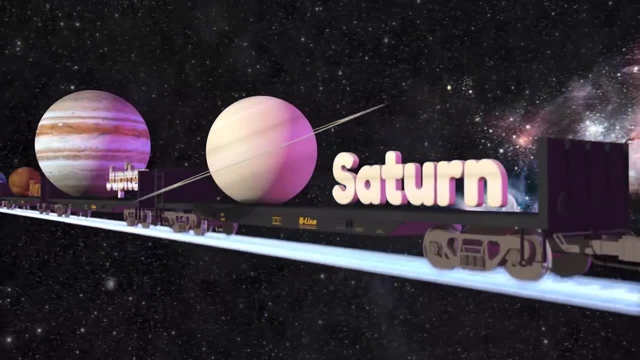 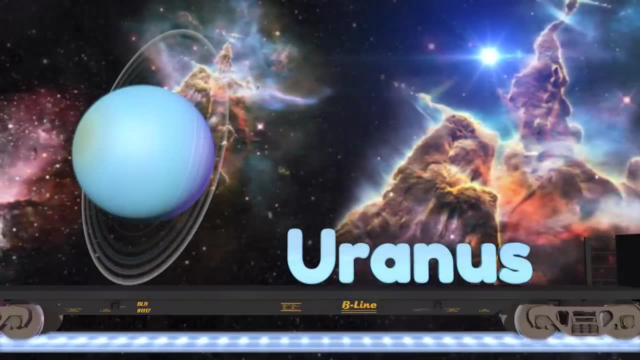 These rings are made up of millions of chunks of rock and dice. Saturn is the second largest gas giant planet. The seventh planet is Uranus, and it has a smaller ring system. Scientists think it may have been hit by an Earth-sized planet a long time ago. 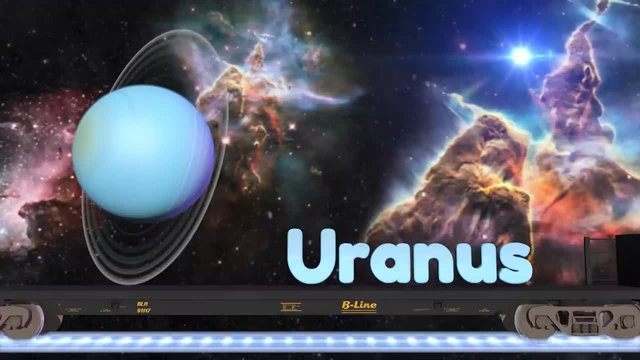 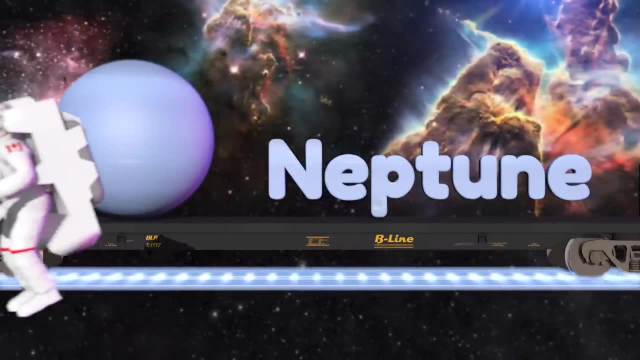 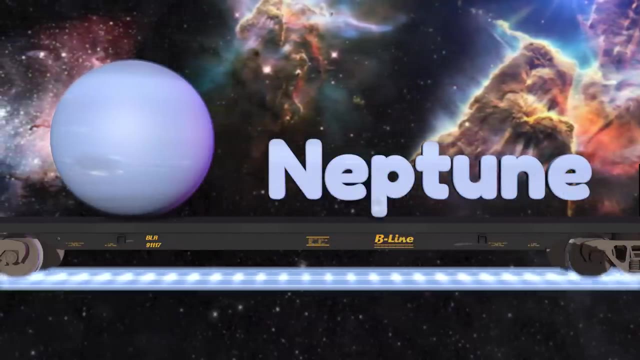 which might be why it's the only planet tilted on its side. The eighth and farthest planet from the Sun is Neptune. Even though Uranus can sometimes reach colder temperatures, Neptune has the coldest average temperature because it's so far from the Sun. 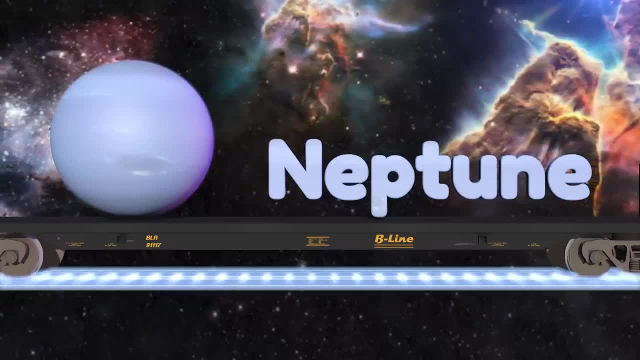 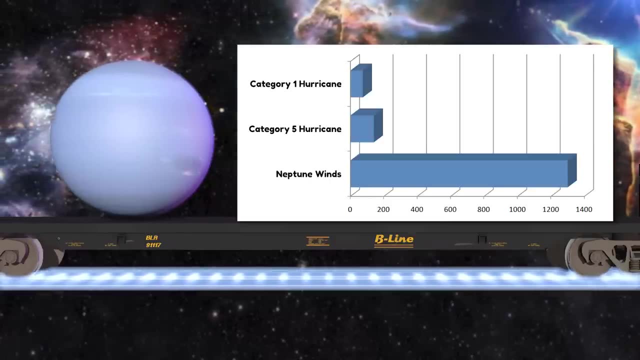 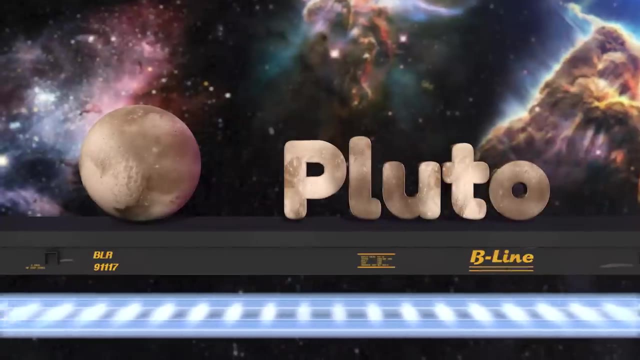 It's also the windiest planet, with winds up to 1300 miles per hour, which is almost ten times as strong as the most powerful hurricanes on Earth. And those are the eight planets in our solar system. There used to be a ninth planet called Pluto. 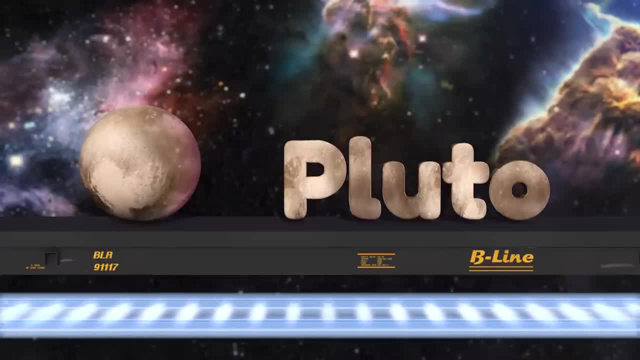 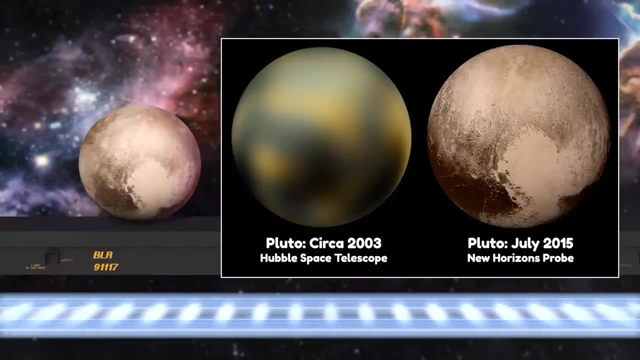 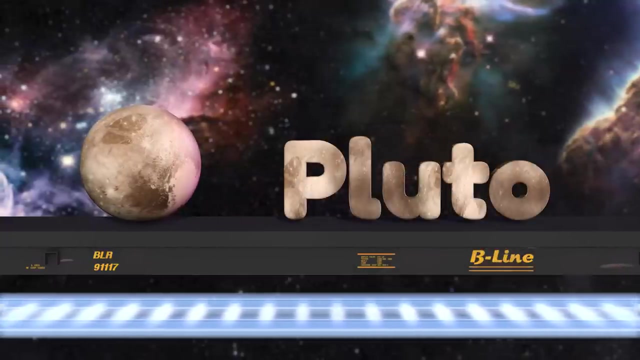 but now it's called a dwarf planet because it's so small, even smaller than Earth's moon. We just got our first high-quality photos of Pluto in the summer of 2015,, when we sent a spacecraft to fly close by. There are at least four other dwarf planets. 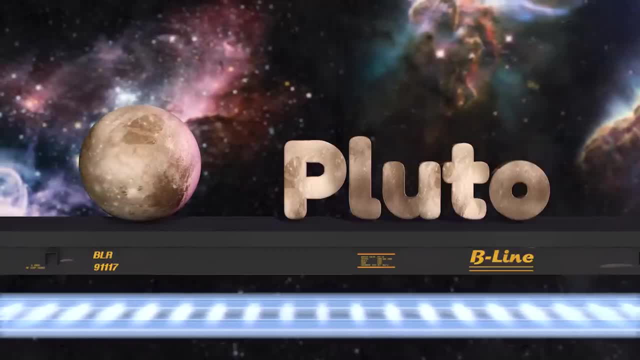 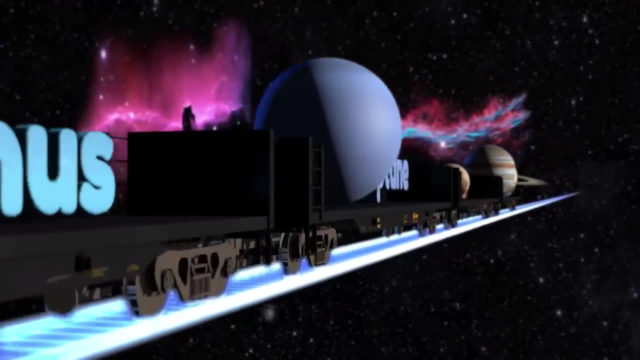 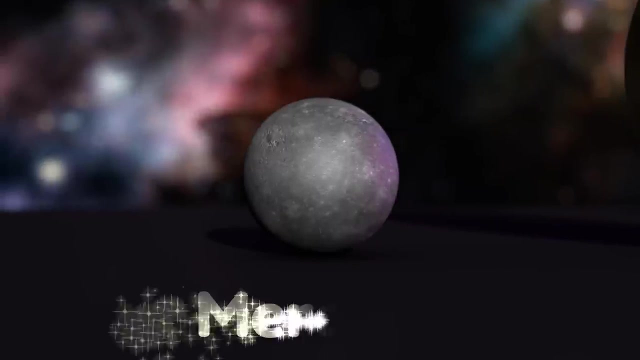 and many more smaller objects in our solar system. There's a big difference in the sizes of the planets. Let's take a look at all eight planets plus Pluto, in their actual scales next to each other There's tiny Mercury, hot and cloudy Venus. 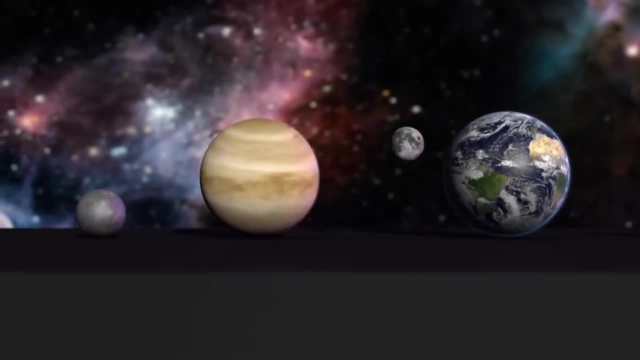 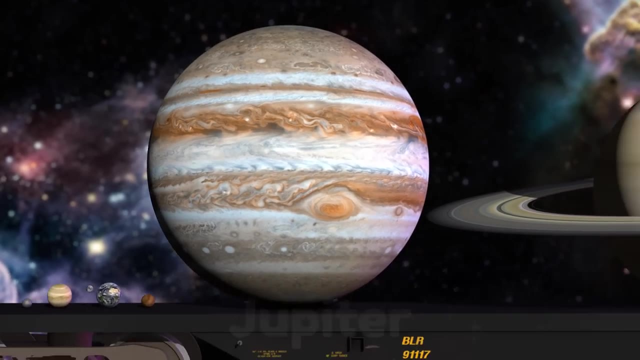 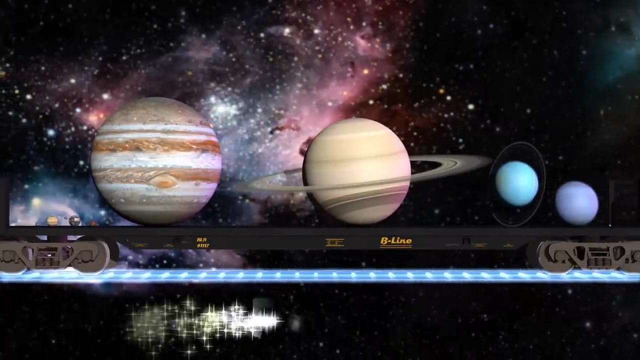 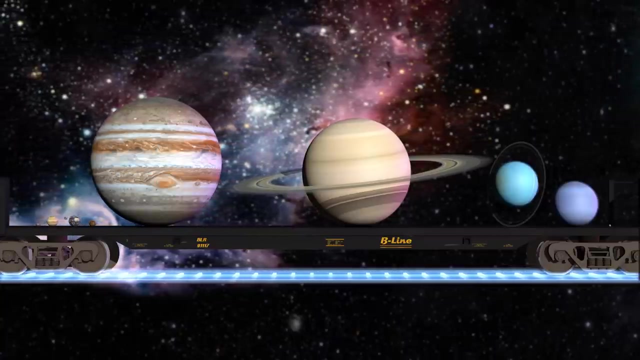 Earth and its moon dusty, Mars, whoa. and there's gigantic Jupiter, Saturn with all of its rings, Uranus and Neptune, and there's the itty-bitty dwarf planet Pluto. But of course, all these planets are tiny when compared to the size of the Sun. 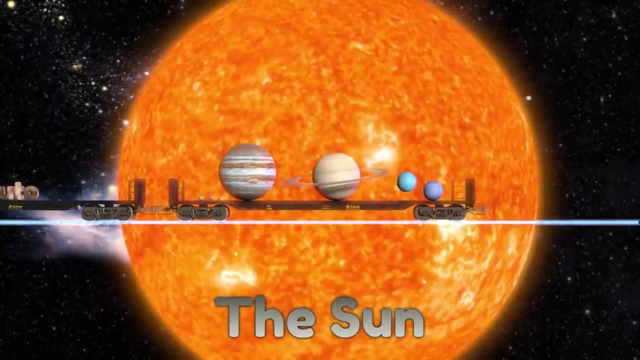 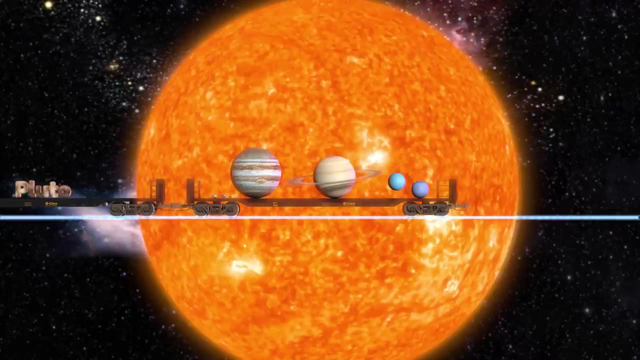 We've learned a lot about the planets over the past hundred years, but we're learning more every day and there's still a lot left to explore. Who knows, maybe one of you will get to visit some of these planets one day. Stay tuned. 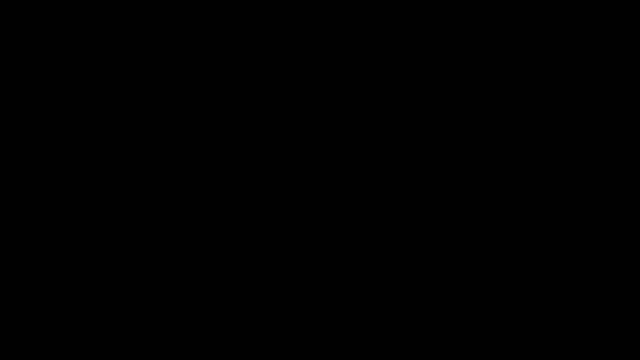 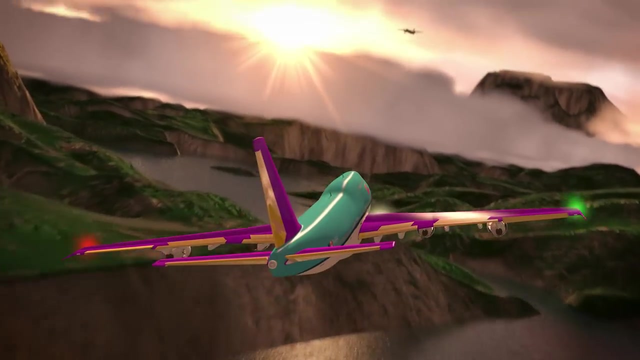 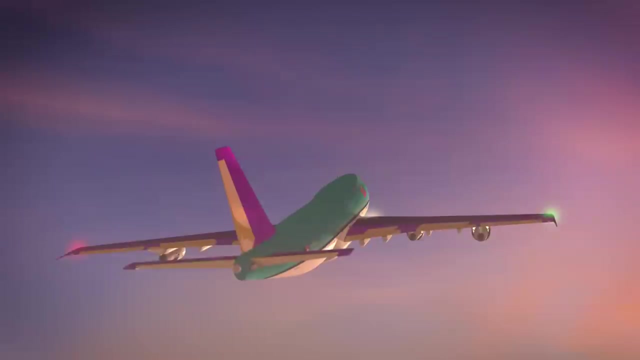 we'll be back after these messages. Hey Brainiacs, Have you ever been for a ride on an airplane? It's so much fun. Airplanes can fly way up in the sky, even higher than the clouds, and they can take you to far off places. 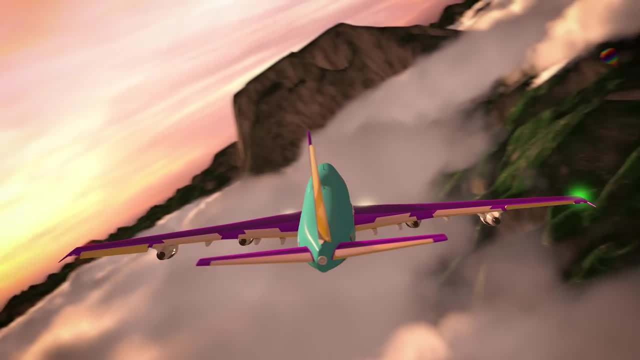 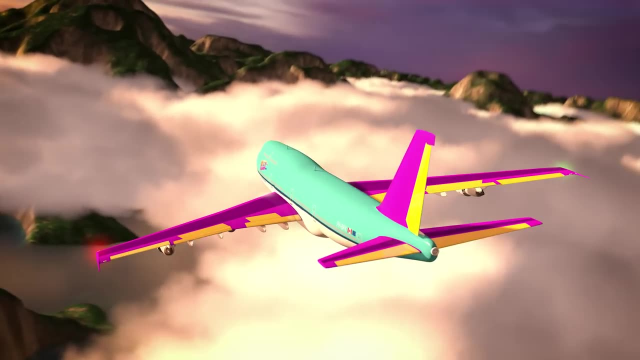 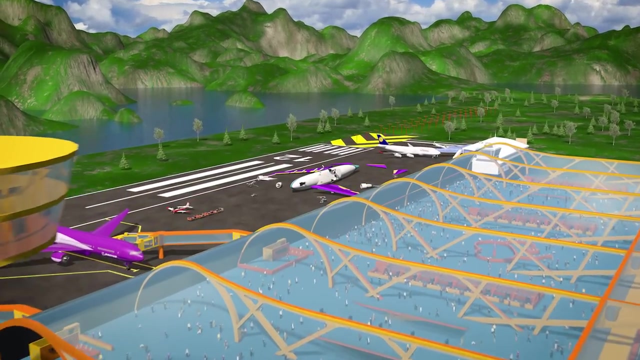 all around the world. Today we're going to learn about the different parts of an airplane and how they work together to make it fly up in the sky. Here we are at the airport where we can find all kinds of cool airplanes. Look all the parts of that airplane. 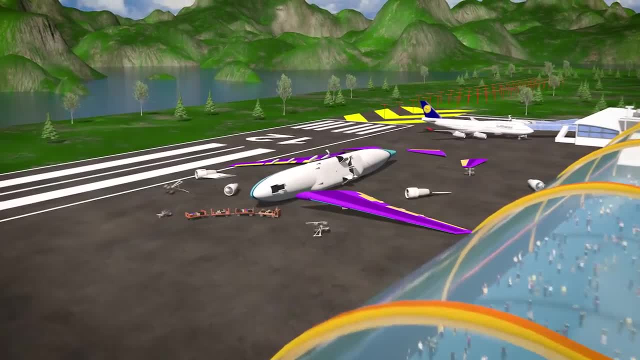 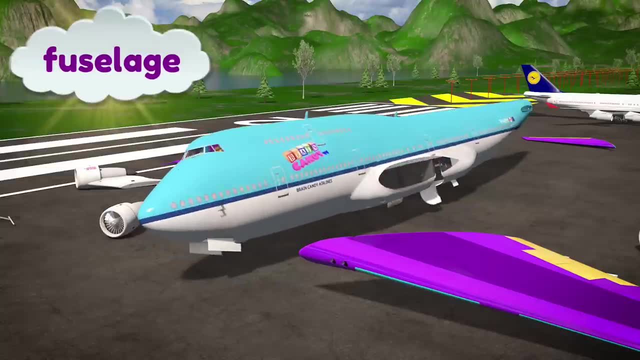 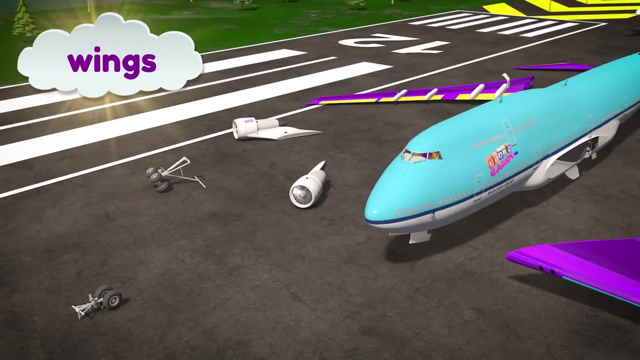 are ready to be put together. Let's see if we can put all the parts in the right spot. The biggest part is called the fuselage. That's where you and all the passengers will sit. Next we have the wings. Do you know which parts are the wings? 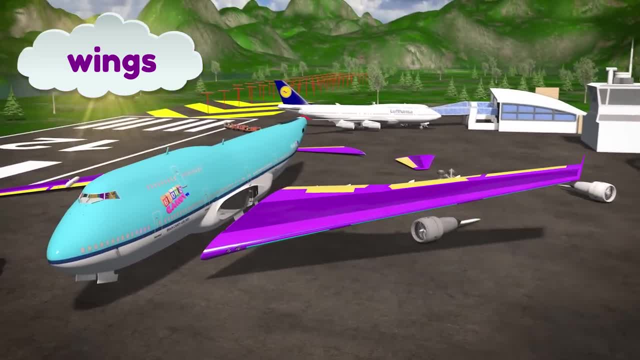 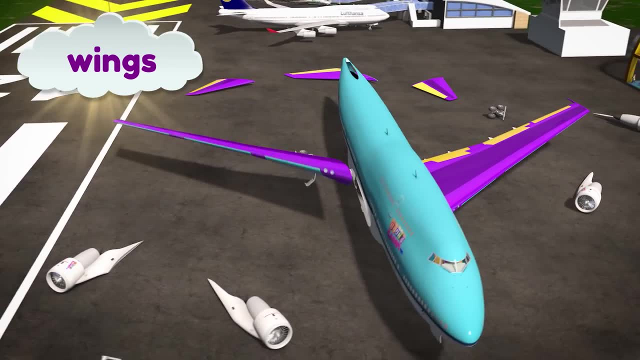 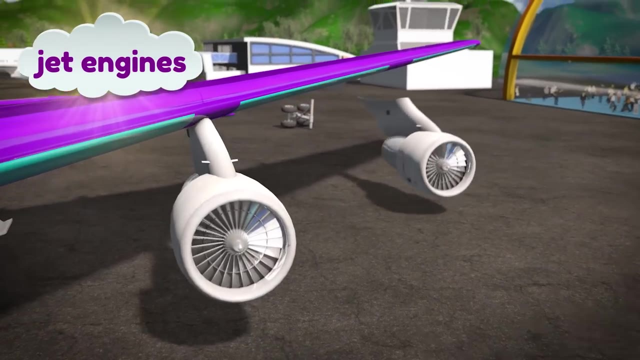 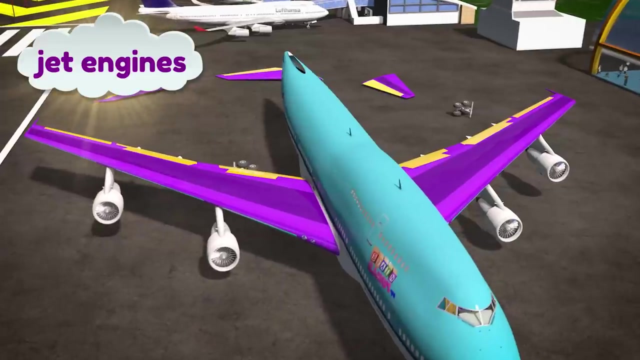 There they are. These wings are a very special shape that helps the airplane fly up through the sky. Under the wings we'll find the jet engines. This big airplane has four engines. The engines push the airplane forward, so it can go really fast. 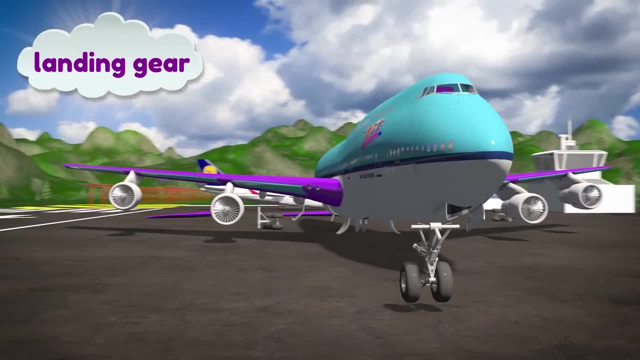 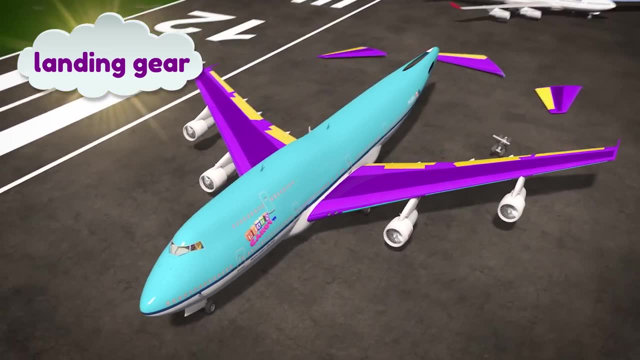 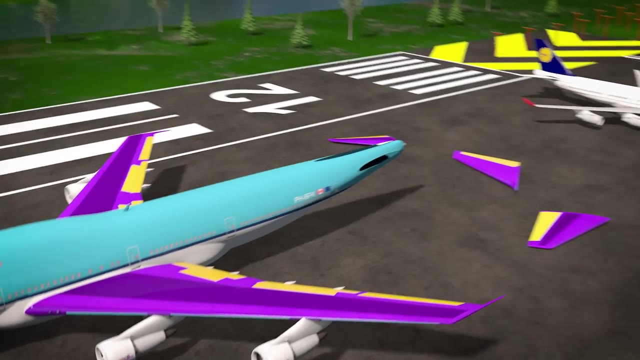 Beneath the wings and fuselage we can find the landing gear. The landing gear has wheels so the airplane can roll along the runway during takeoff and landing. At the back of the airplane we'll find the stabilizers. These stabilizers help keep the airplane flying straight. 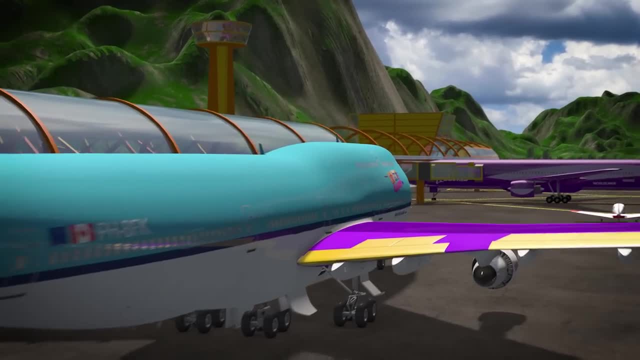 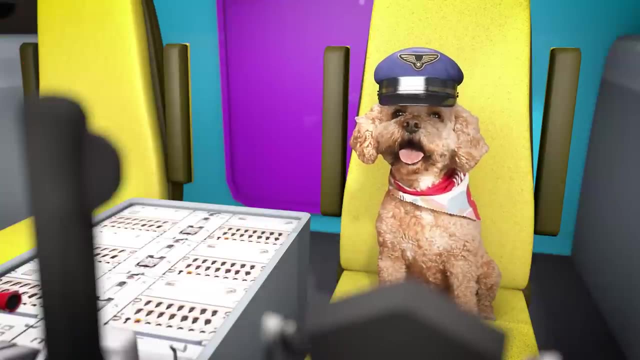 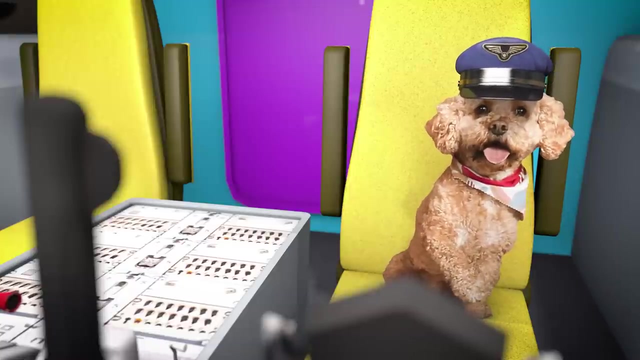 Now that our airplane is all put together, let's hop on board and learn how it works. Hey, Captain Lizzy, Are you ready to take us for a ride on this new airplane? Alright, Here we are, at the front of the airplane, And this area is called the flight deck. 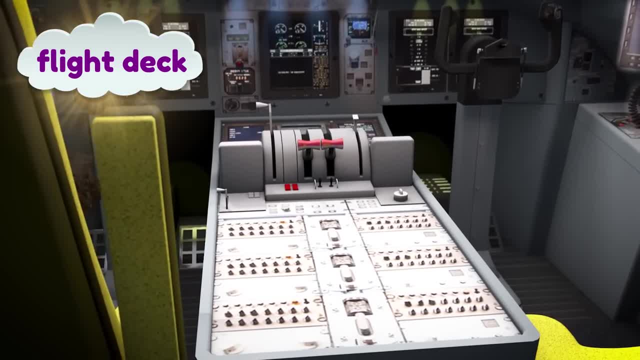 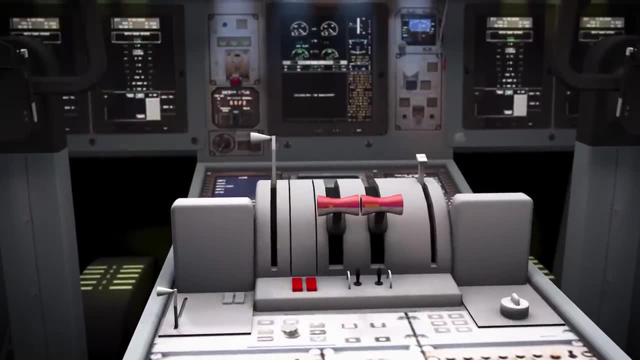 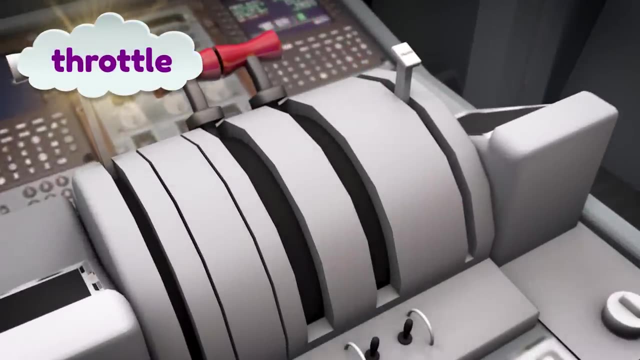 The flight deck is where the captain sits and controls the plane. Let's explore the flight deck and learn some of the things the captain uses to control the airplane. This is the throttle. The throttle controls the thrust of the engines. That's what makes the airplane go faster or slower. 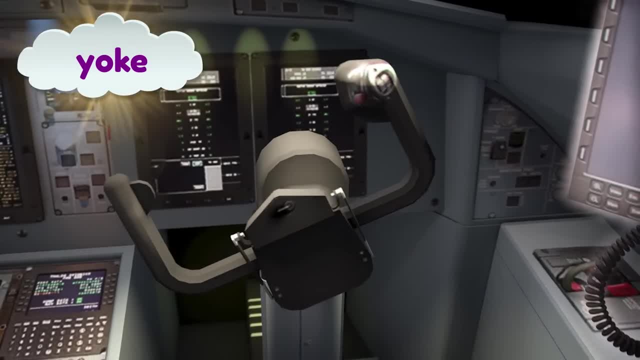 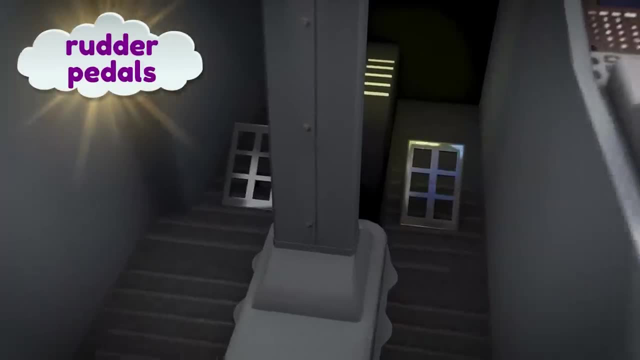 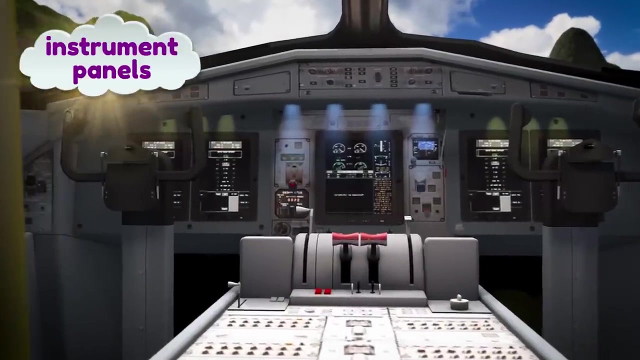 Here is the yoke. The yoke is like the steering wheel of an airplane. The rudder pedals found here also help Captain Lizzy steer the airplane. The instrument panels have lots of buttons and screens to give the pilot information about where to go. 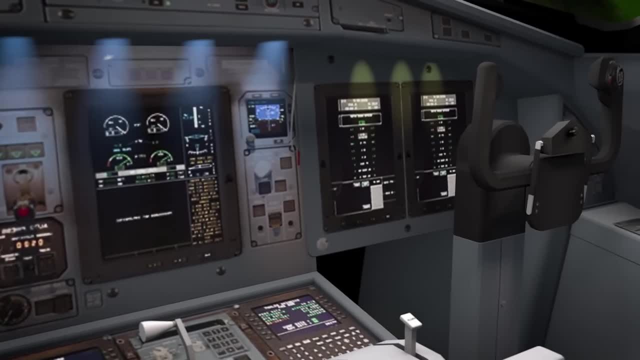 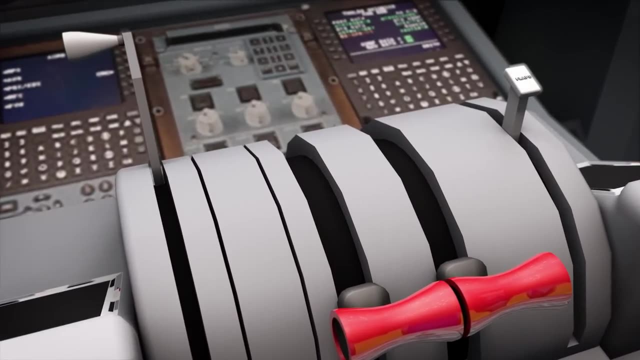 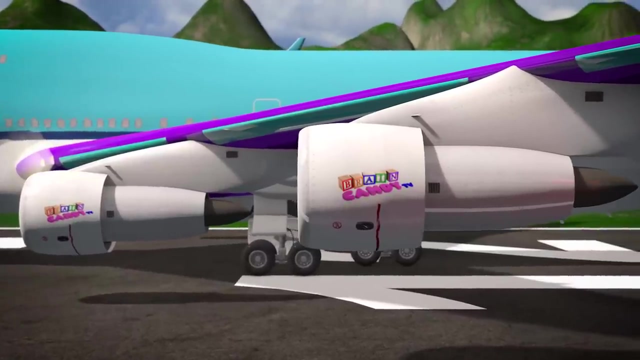 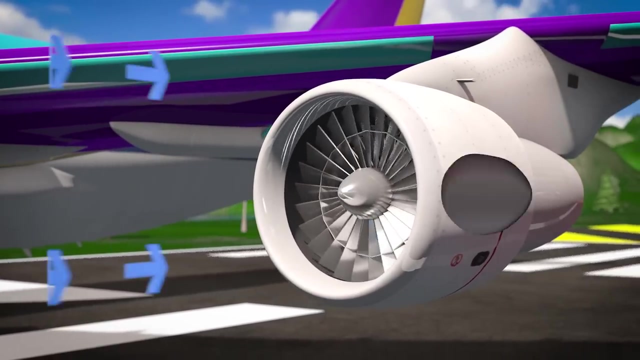 and how the airplane is flying. Alright, Let's get those big jet engines going and get ready for takeoff. Give it some throttle Lizzy. These are powerful turbofan jet engines. Let's learn how they work. These engines use a series of fans. 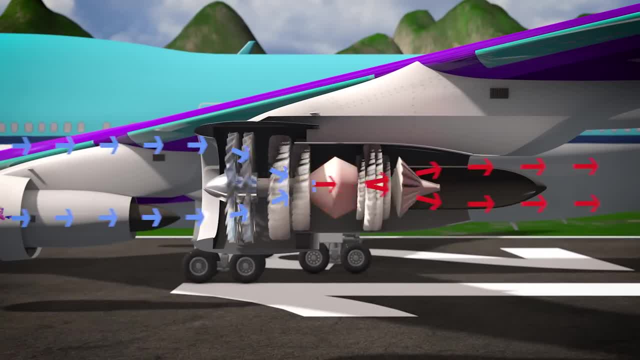 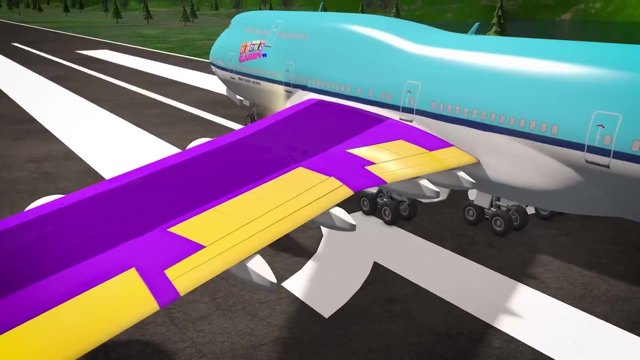 to squeeze the air smaller and smaller. Then they add jet fuel to the squeezed air and explode it, shooting the hot air out the back and pushing the airplane forward. The big parts at the back of the wing are called flaps. When the flaps move down, 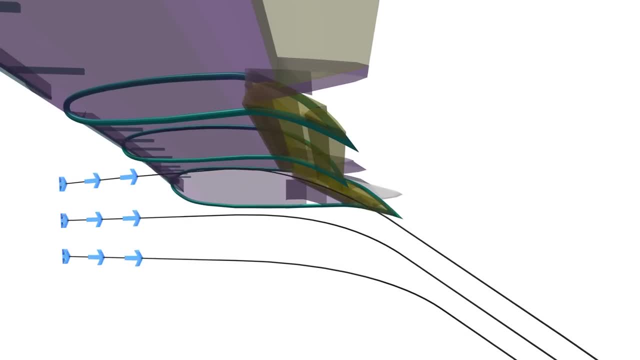 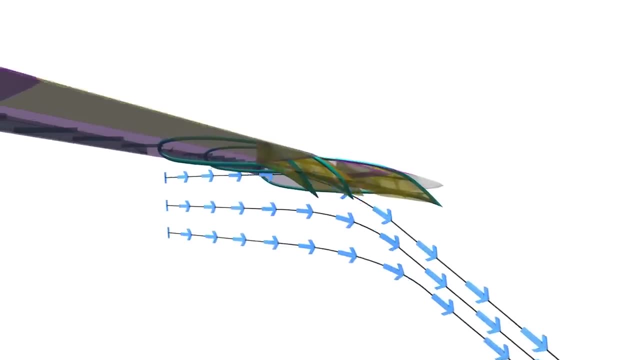 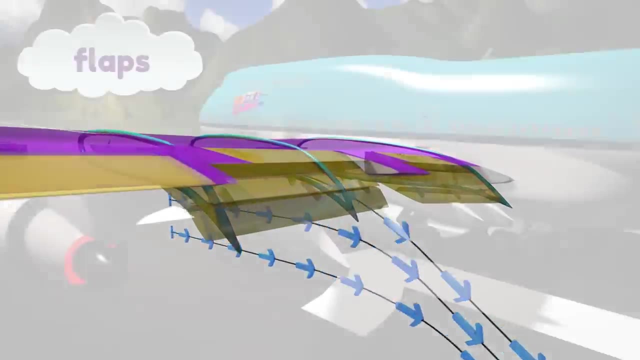 they create extra lift by squeezing the air under the wings as the airplane moves forward quickly through the sky. This squeezing of the air pushes the airplane up. The flaps also create drag which slows the airplane down These parts at the front of the wings. 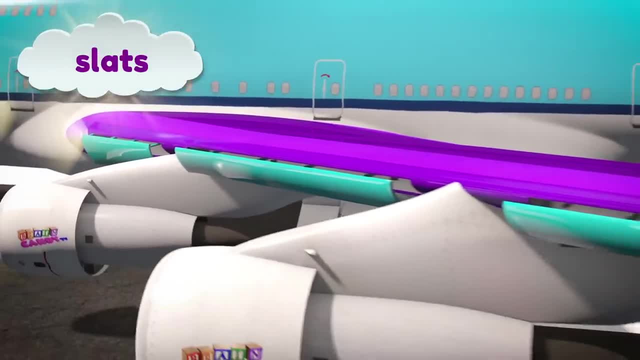 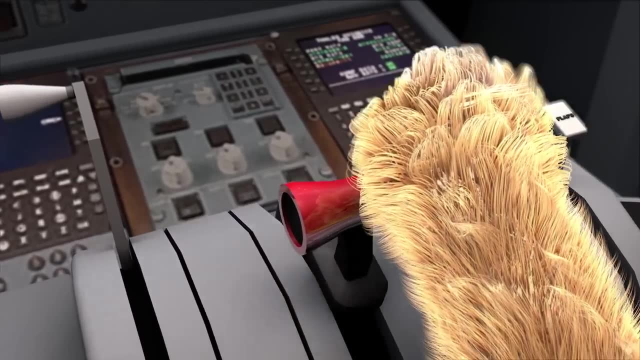 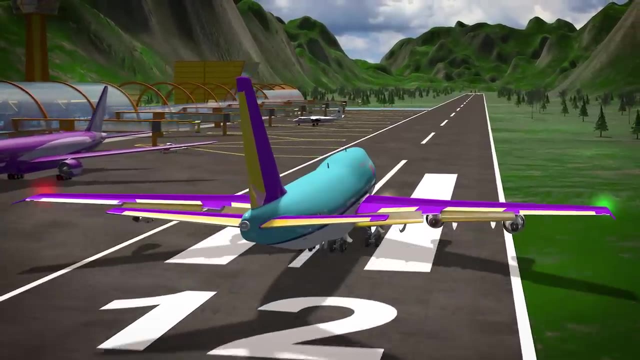 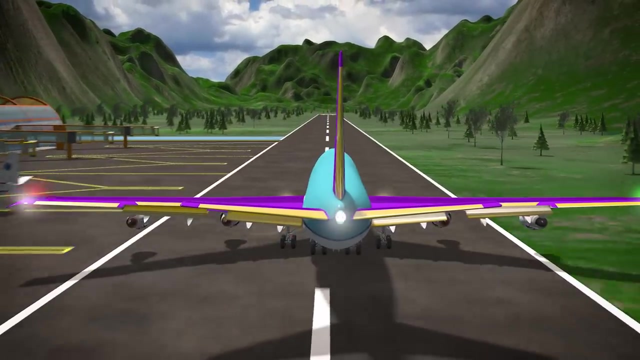 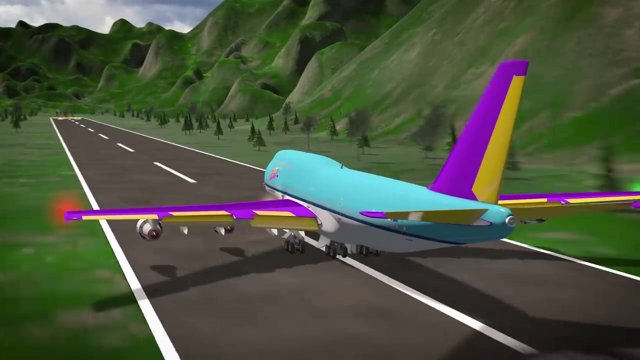 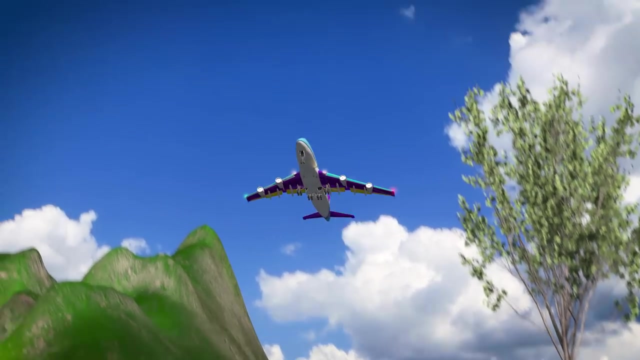 are called slats. They're used to create even more lift, which pushes the airplane up in the air. Okay, Lizzy, give it full throttle Time for takeoff. All right, Now that we're high up in the sky, we can retract the landing gear. 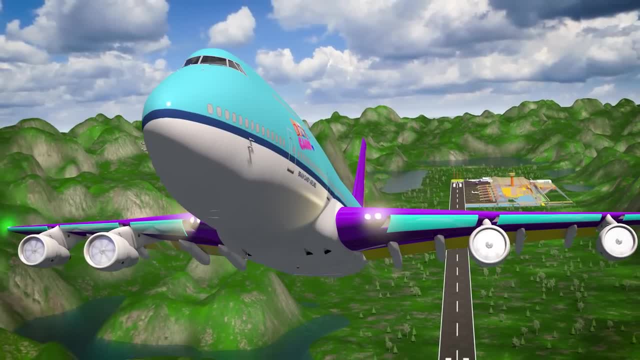 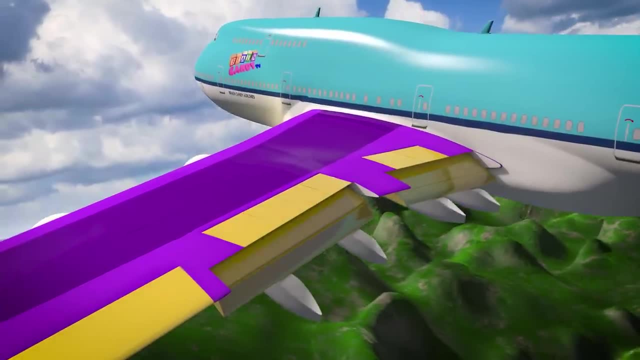 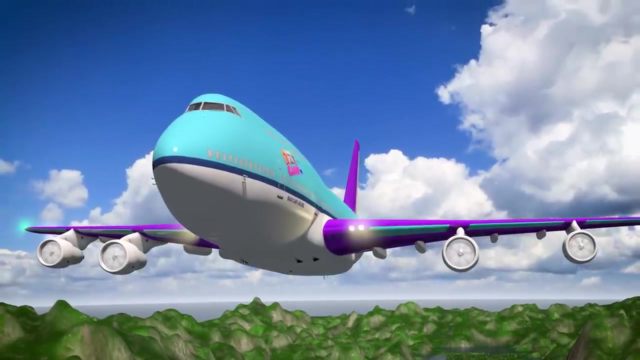 so the airplane can go even faster. We don't need as much lift, so we can now close the slats and raise the flaps. Now let's learn about all the moving parts that Captain Lizzy can use to steer the airplane through the sky. 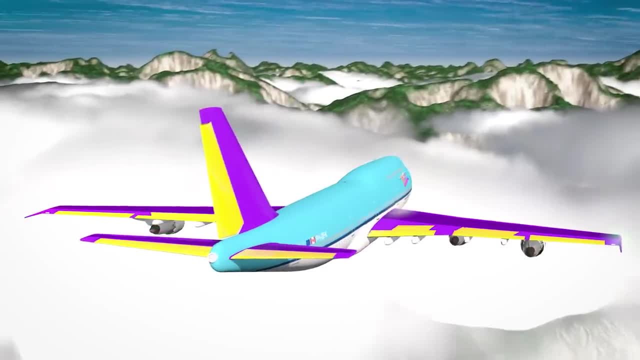 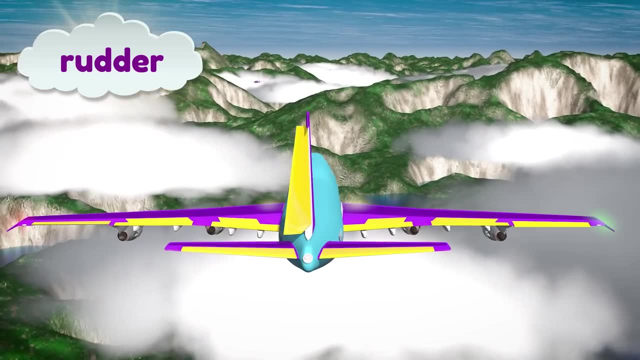 If Captain Lizzy wants to turn the airplane left or right, she'll use this part called the rudder. It works just like a rudder on a sailboat: When the rudder moves to the left, the airplane turns to the left. 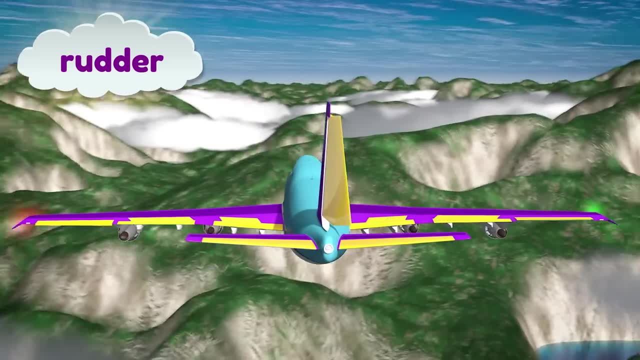 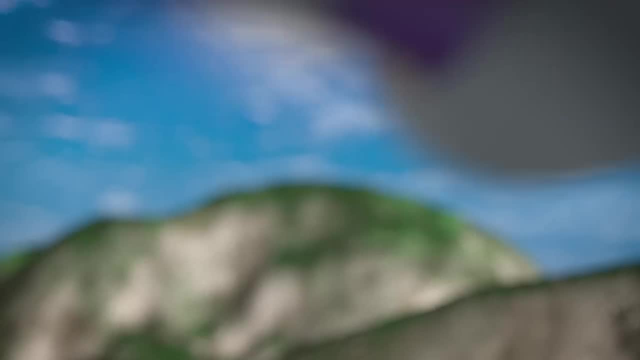 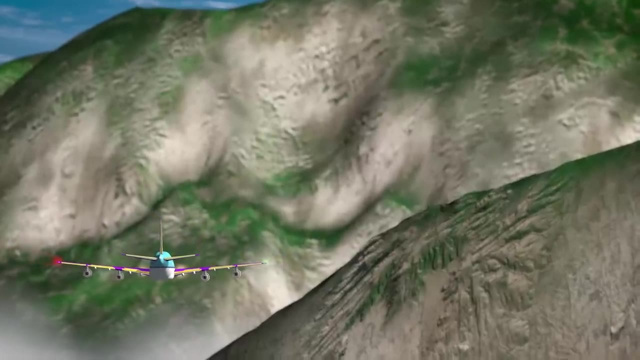 When the rudder turns to the right, the airplane turns to the right. Oh no, look, We're heading right for that big mountain. We need to get higher in the sky To pitch the airplane up or down. we'll use these parts at the back of the plane. 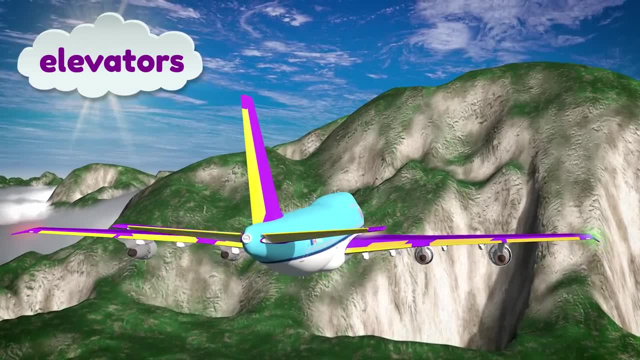 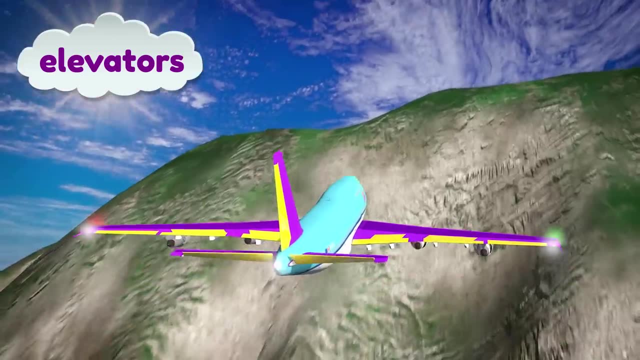 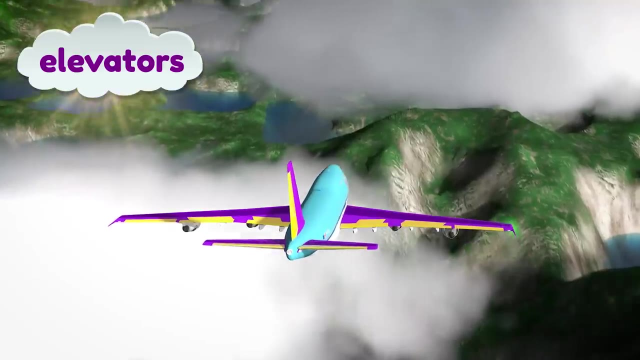 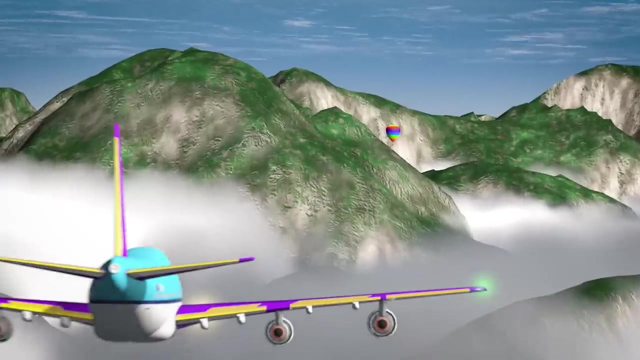 called the elevators. When the elevators move up, the nose of the airplane moves up. Hurry Lizzy, We're getting really close to that mountain. Phew, that was a close one. Hey, what's that hot air balloon doing way up here? 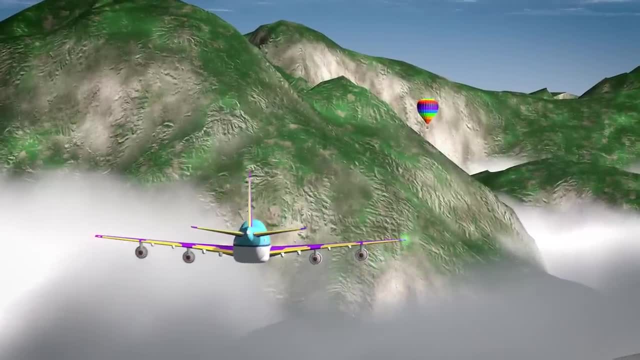 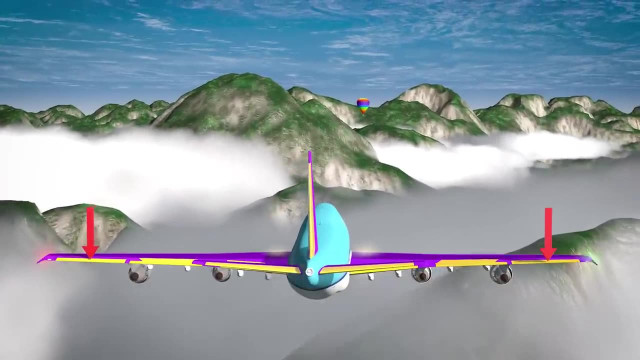 We better make a quick turn to get around it. If we want to roll the plane for an even faster turn, we'll use these small parts at the ends of the wings. These parts are called ailerons. When one aileron goes up, 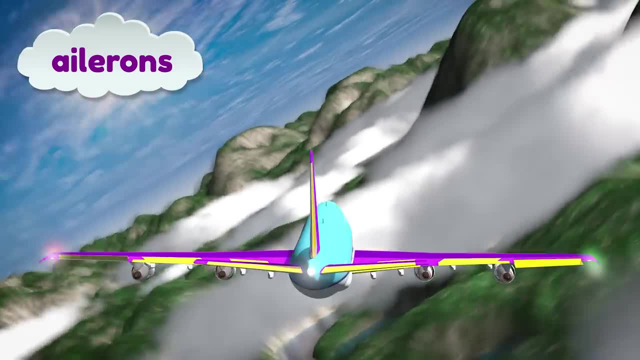 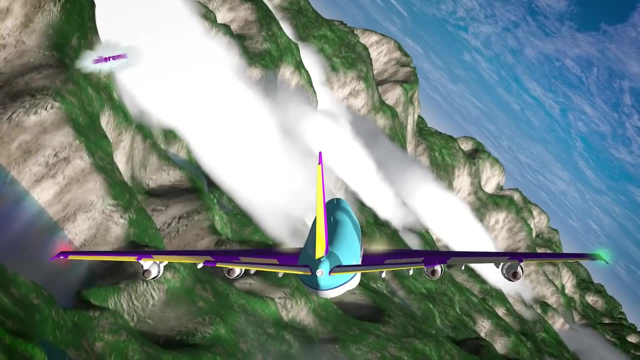 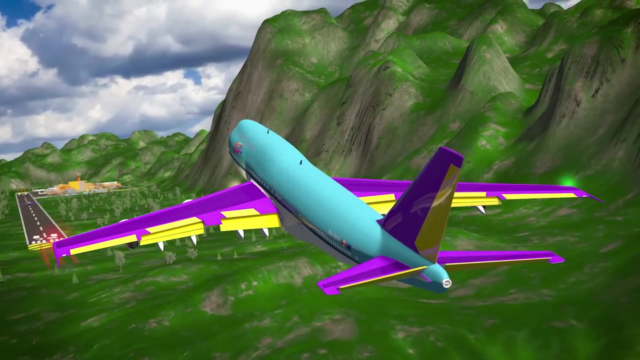 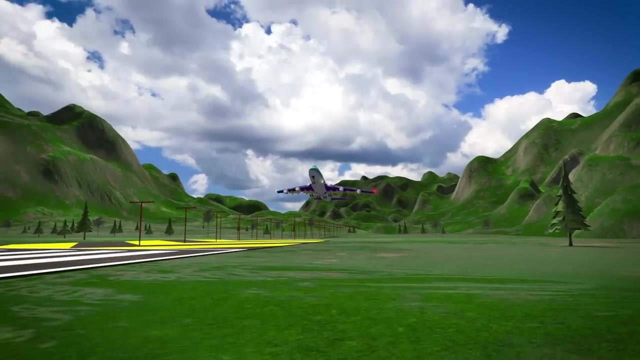 the other one goes down, causing the airplane to roll. OK, Captain Lizzy, our flight is almost done. Time to bring it in for a landing. When Captain Lizzy wants to slow the airplane down before landing, she'll use these parts on the top of the wings. 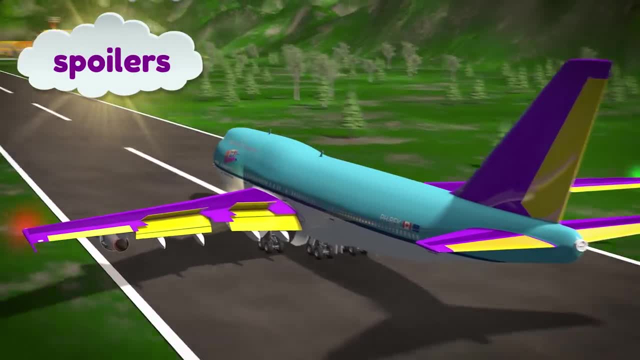 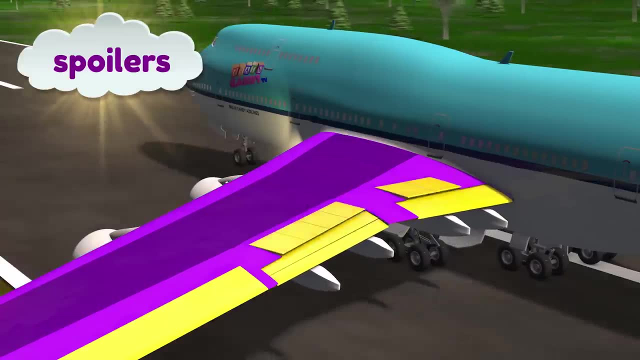 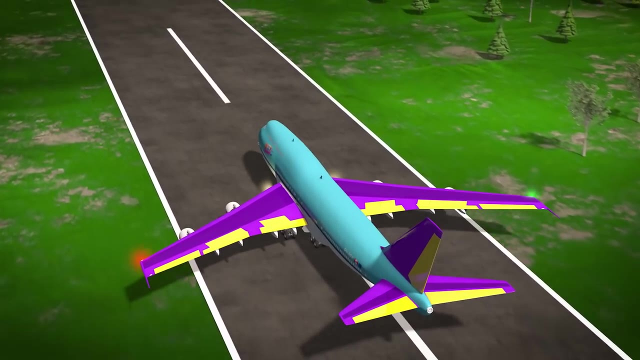 called spoilers. When the spoilers are used along with the slats and the flaps, this will slow the airplane down for a nice, smooth landing. Nice landing, Lizzy. Great job, Brainiacs. Now you know a lot about airplanes and how they work. 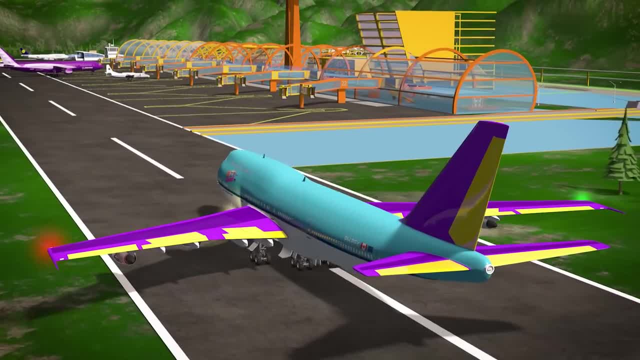 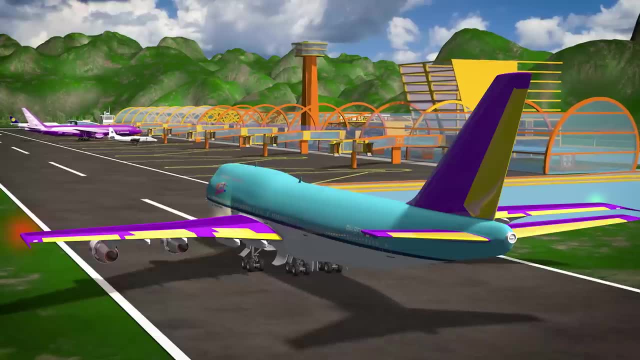 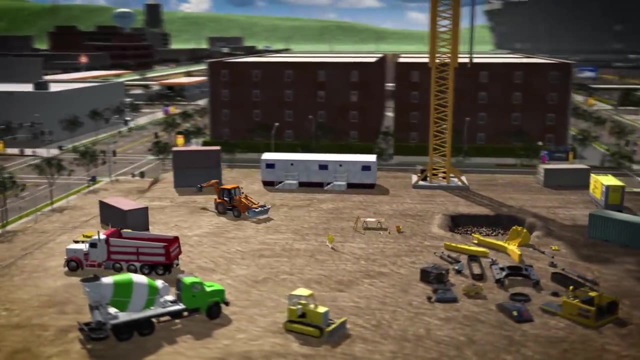 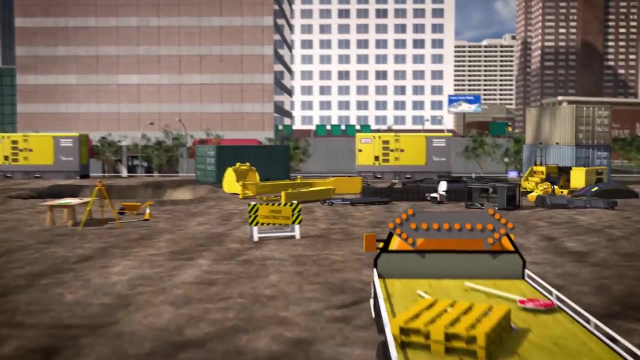 Aren't airplanes cool? Learning how things work is so much fun. What do you want to learn about next? Hey Brainiacs, Check out this big construction site. Wow, Look at all the awesome construction vehicles. Do you know what an excavator is? 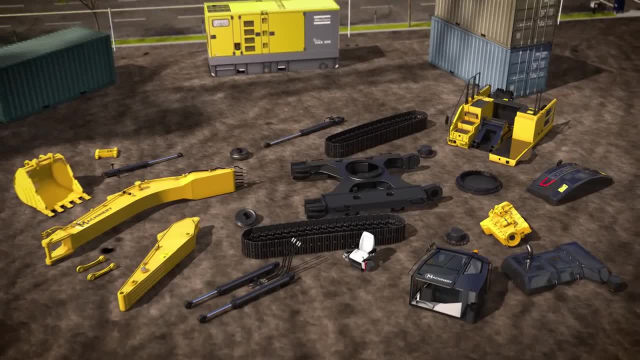 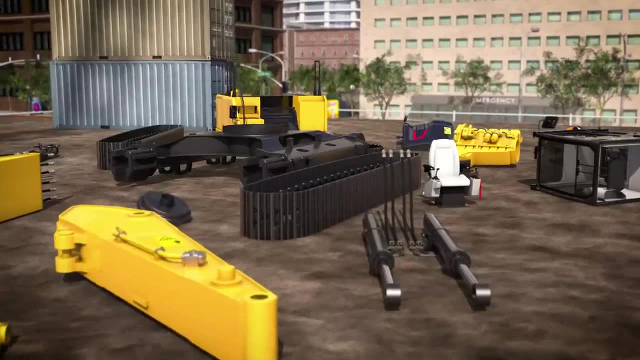 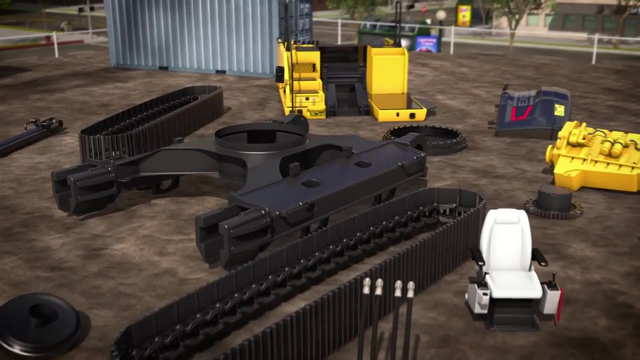 They're so cool. They use something called hydraulics, which makes them super strong and really good at digging holes. Let's put this excavator together from all the different parts so we can learn how it works. First, we have this big part called the chassis. 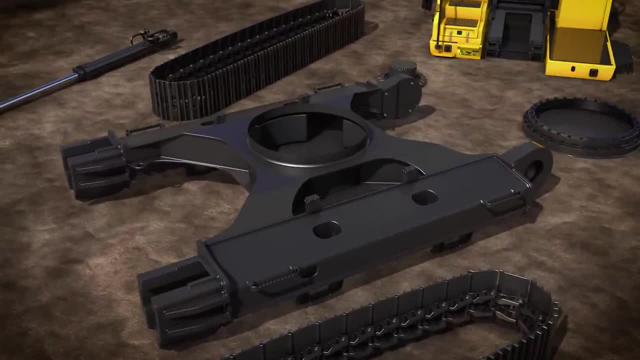 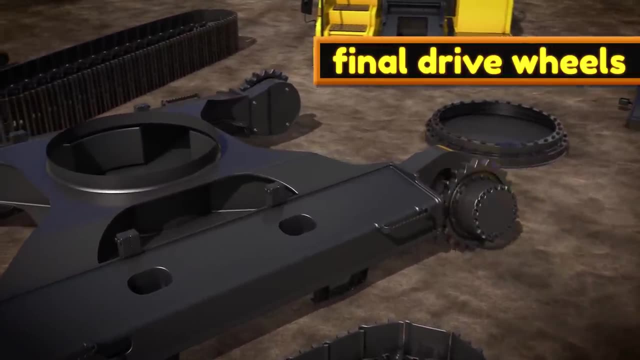 which holds the bottom parts together. Now let's add the final drive wheels. The final drive wheels have bumpy sprockets which will be used to move the tracks. At the other end of the chassis we'll find the front idler wheels. 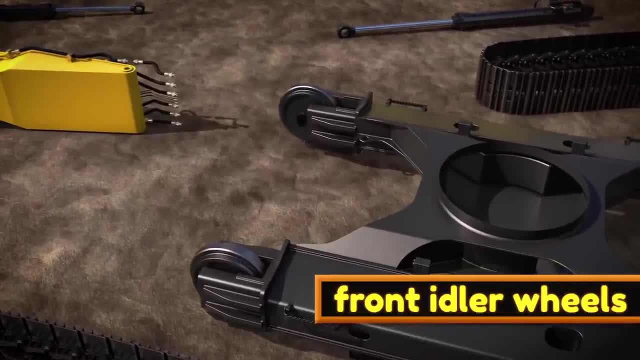 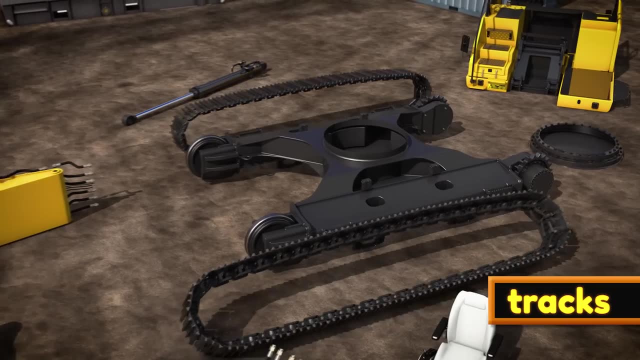 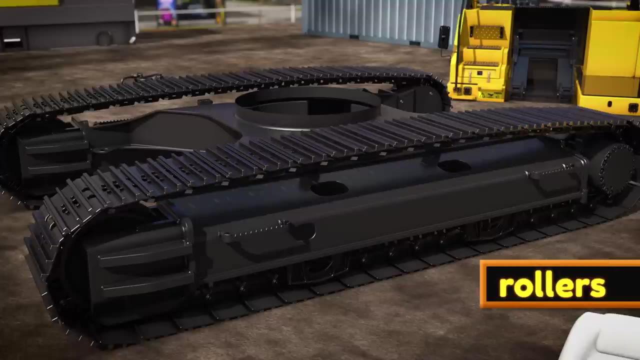 These wheels help the track roll around the front of the chassis. Now we'll add the tracks to the chassis. These tracks give the excavator lots of grip so that it can drive over bumpy ground and mud. Then we'll need some rollers at the top. 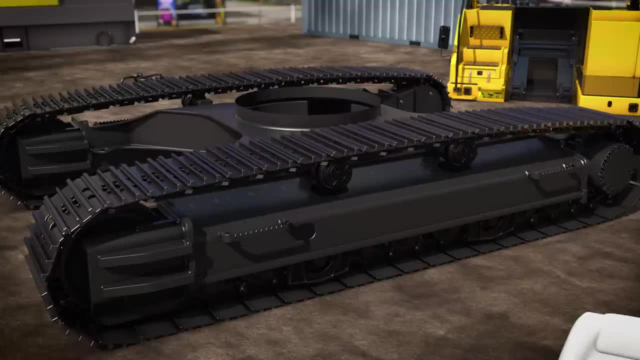 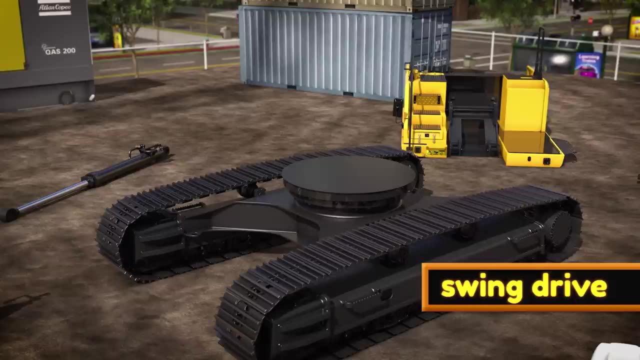 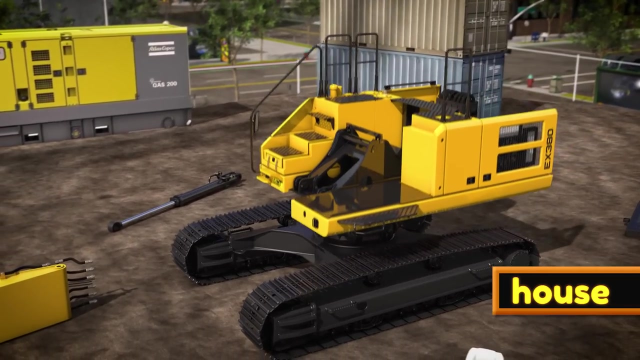 and at the bottom for the track to roll along. On top of the chassis is the swing drive. The swing drive allows the excavator to spin around quickly. This big part is called the house. The house holds the engine and connects all of the upper parts together. 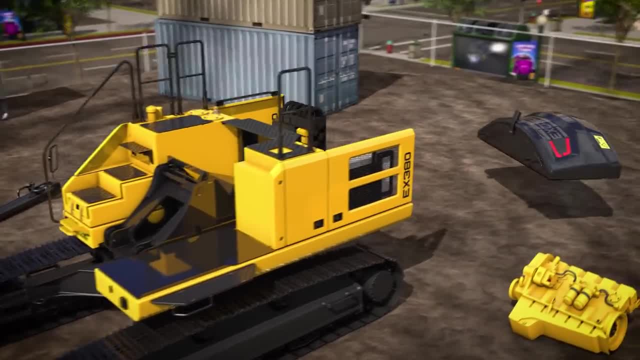 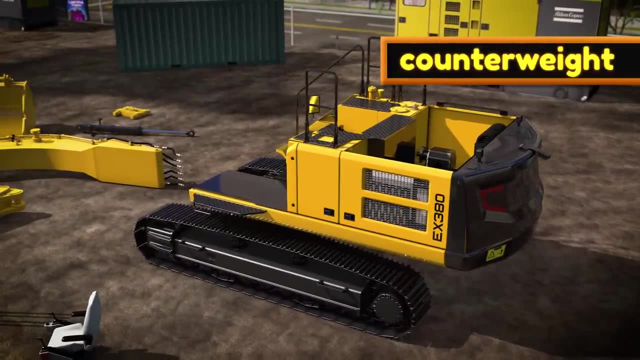 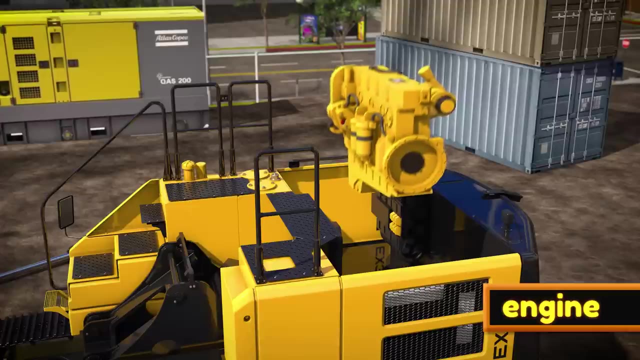 On the back of the house there's a big heavy piece called a counterweight. This helps keep the excavator balanced when it's digging with its big arm at the front. Now we'll add the engine. That's the part that provides power to the excavator. 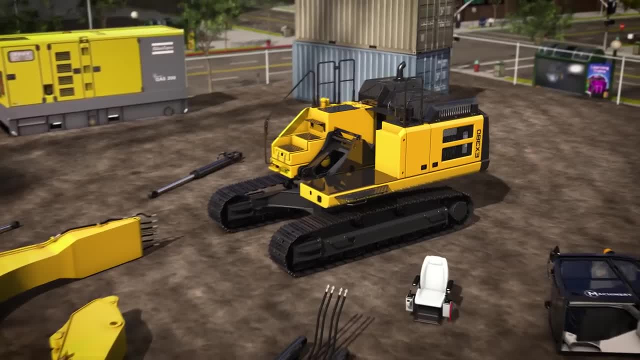 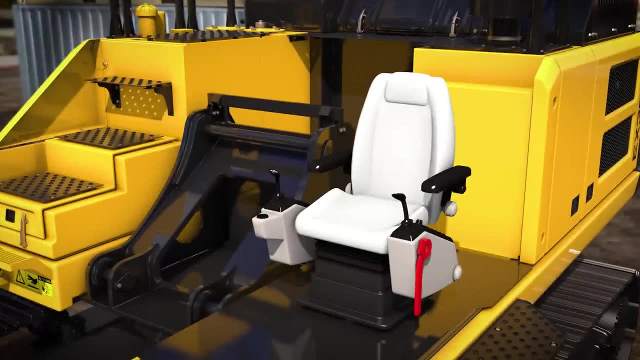 and makes everything move. Let's add a seat so the operator has somewhere to sit. On either side of the seat there are two joysticks. The operator uses these joysticks to control the big arm of the excavator. This part is called the cab. 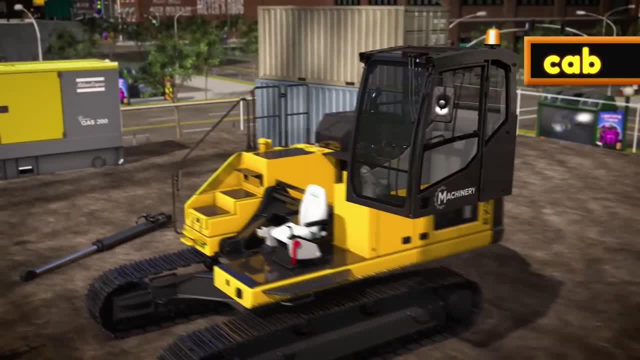 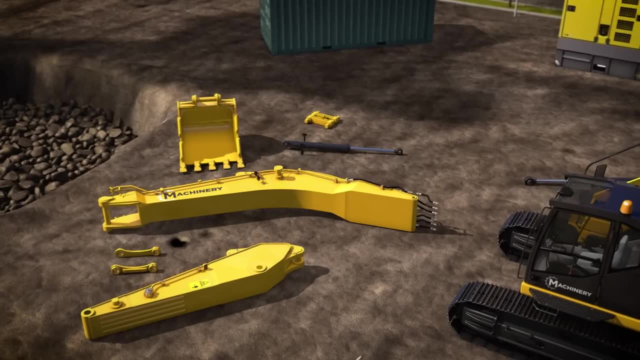 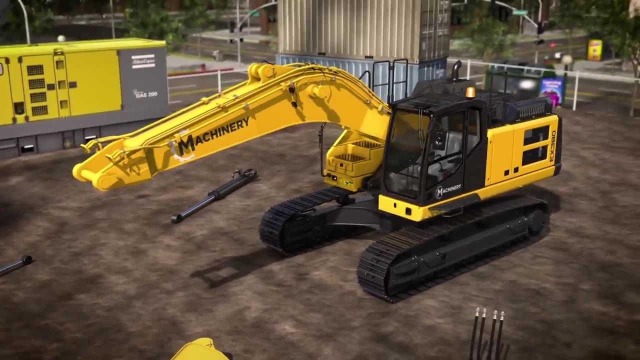 It keeps the operator safe at the dangerous construction site. Now it's time to assemble the big arm of the excavator. This big, strong part is called the boom. Beneath the boom we'll add the hydraulic boom cylinders. These parts can move the boom up and down. 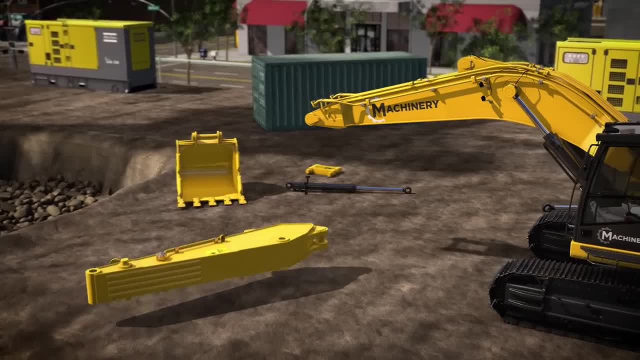 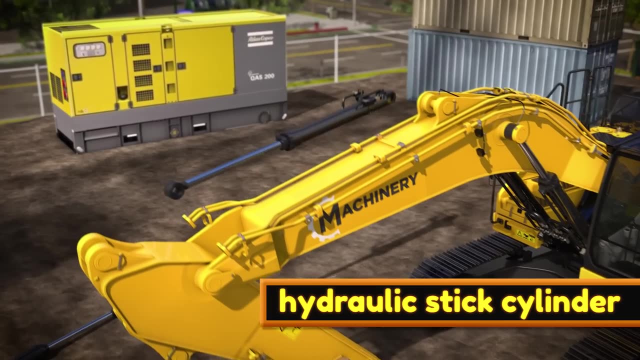 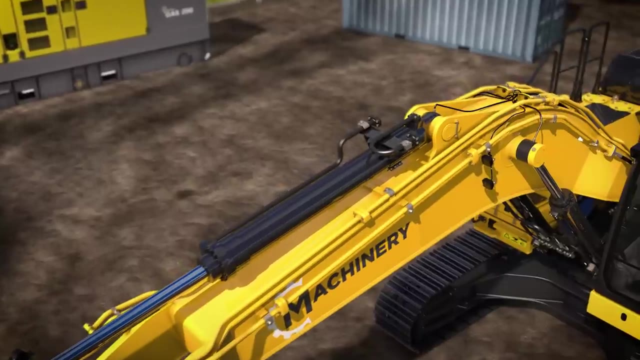 with amazing strength. The next part of the big arm is called the stick. Now we need to add the hydraulic stick cylinder. This will push the end of the stick in or out. The stick cylinder needs to be connected with hydraulic hoses. One hydraulic hose goes to the front of the cylinder. 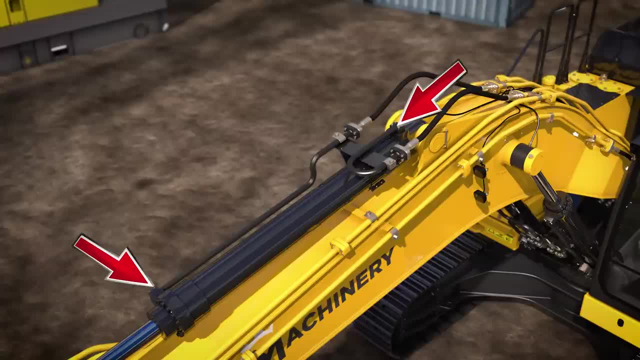 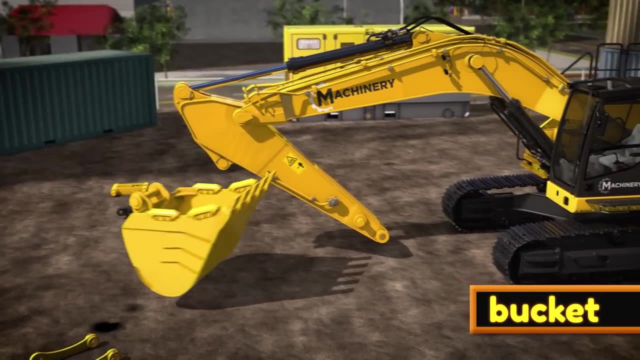 and one goes to the back. We'll see why this is important later. At the end of the stick we have the bucket. The bucket is the part that helps the excavator dig deep holes and lift lots of rocks and dirt The pointy teeth at the end. 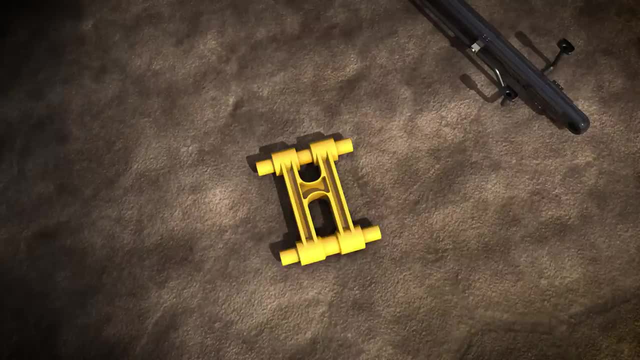 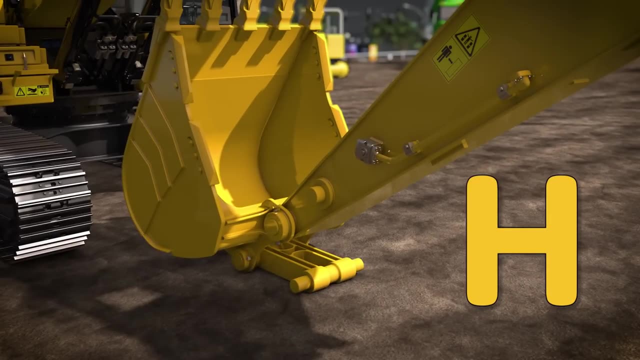 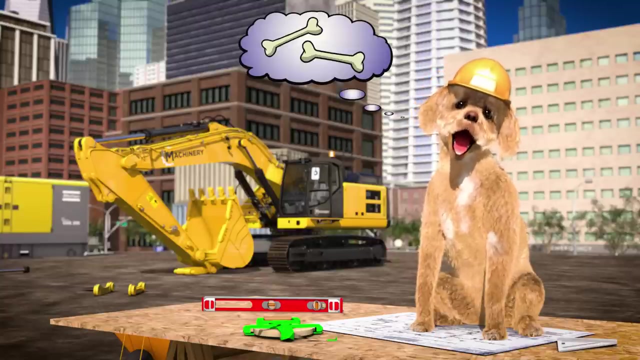 help the bucket cut into the hard ground. This part is called the H-link because it's shaped like a capital letter H. These parts are called dog bones. Don't get too excited, Lizzy, They're just shaped like dog bones. But you wouldn't want to chew on these? 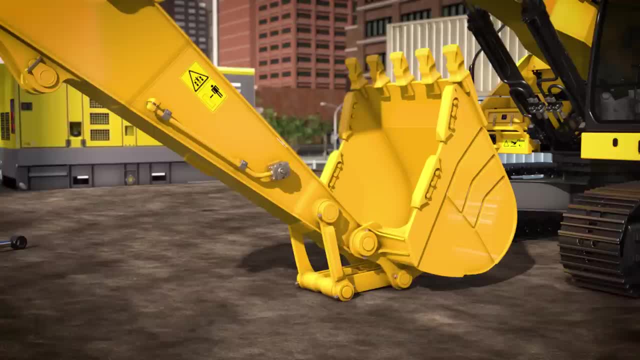 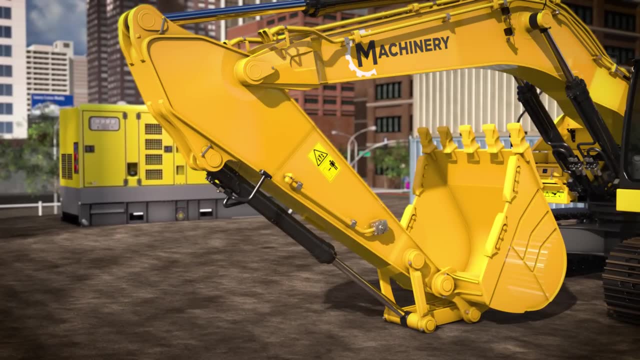 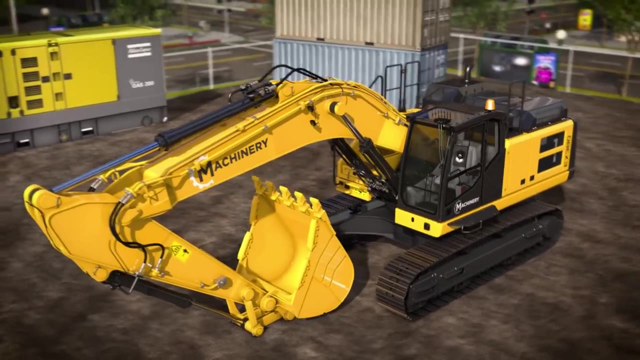 The dog bones are used to connect the H-link to the stick. Finally, we'll add the hydraulic bucket cylinder to connect to the H-link, along with more hydraulic hoses so we can control the bucket. Awesome, Our big, powerful excavator is now complete. 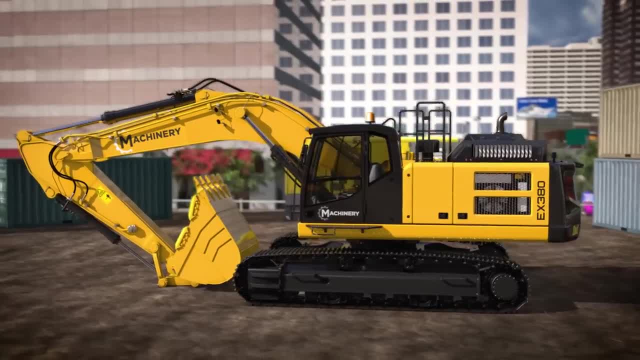 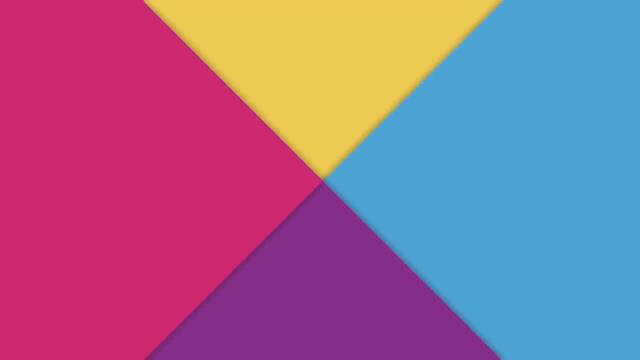 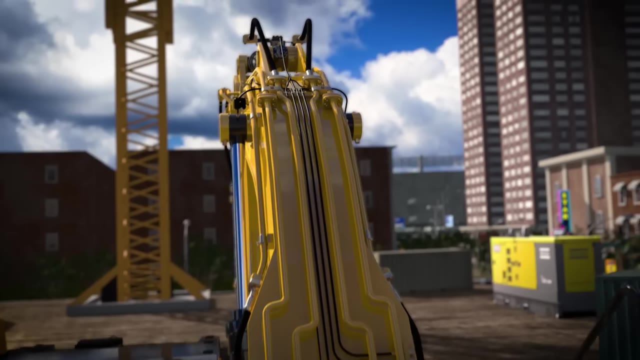 Do you want to know the secret to why excavators are so strong? It's something called hydraulics. Let's learn how it works. Inside the excavator there is a pump that pushes hydraulic fluid, like engine oil, really quickly through small tubes. 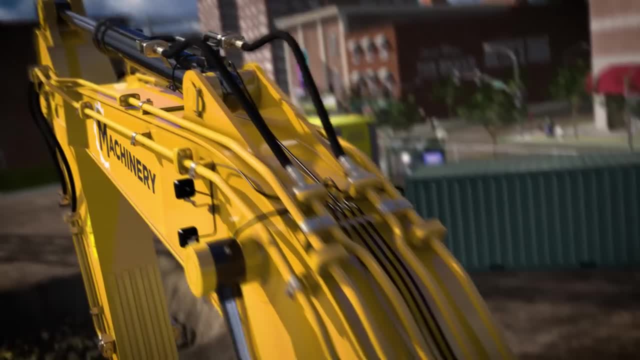 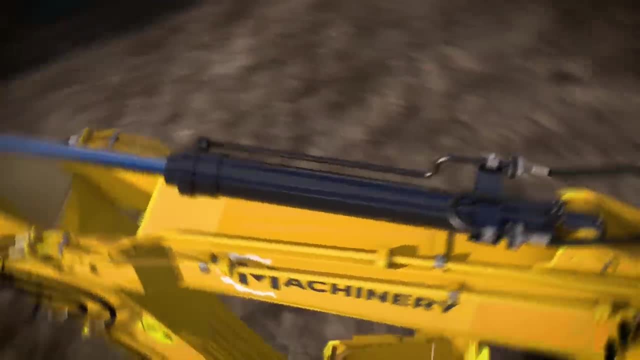 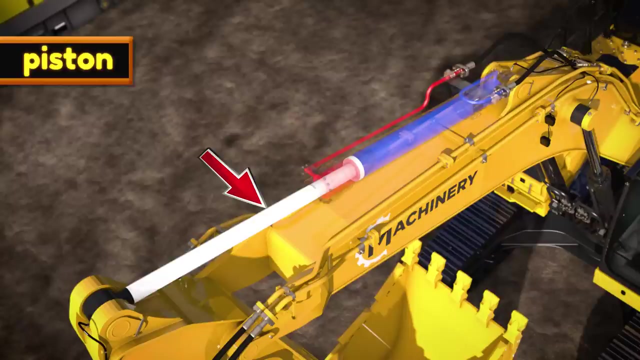 The fluid then goes into one end of a hydraulic cylinder. here or here Inside the cylinder, there is a piston which separates the fluid coming in from each end of the cylinder. If you want the piston to come in, you pump the fluid shown in red. 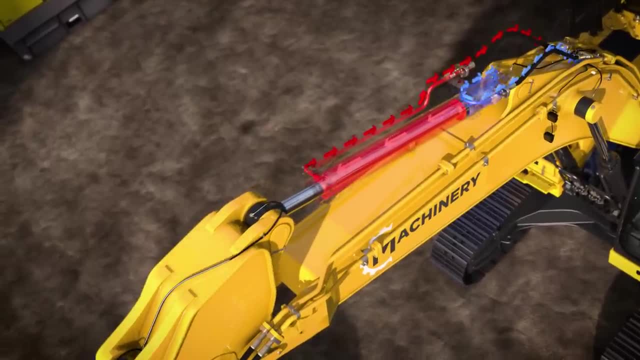 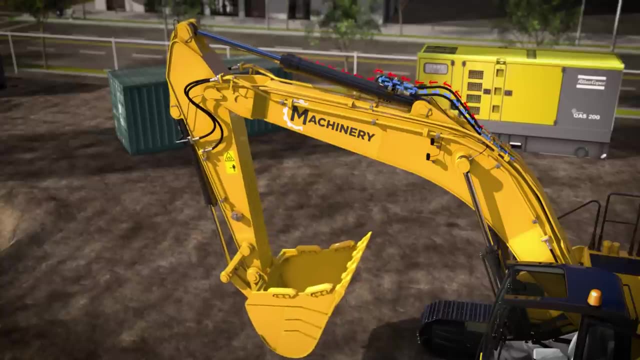 into this end. If you want the piston to go out, you pump the fluid shown in red into the other end. When the high speed fluid from the tubes moves into the much wider cylinder it slows down but it pushes against the piston. 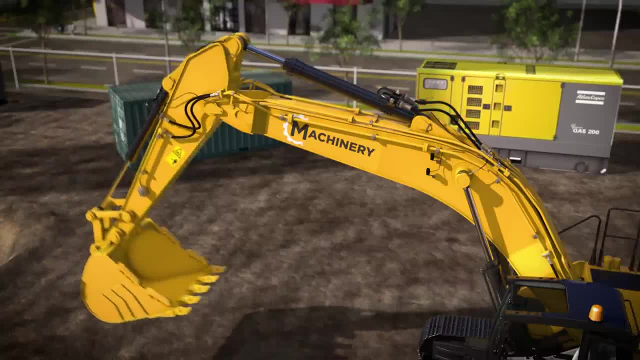 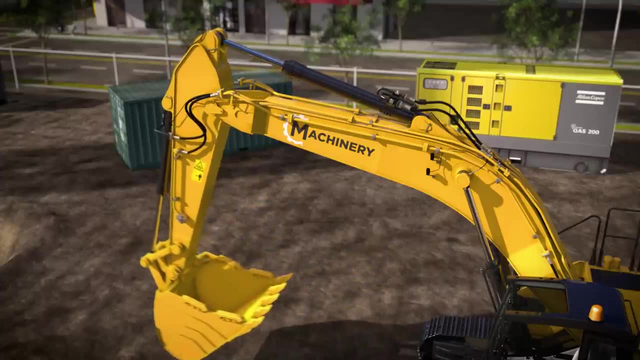 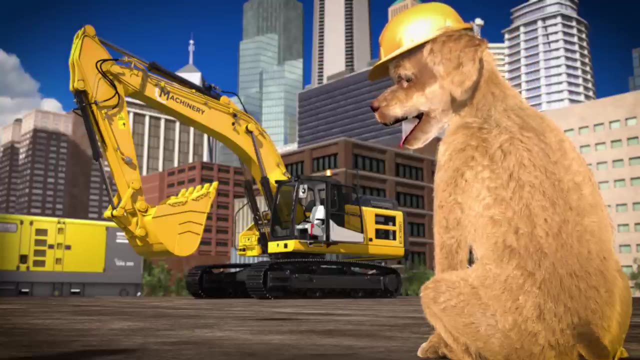 with much greater force. So by controlling the fluid going into each end of all the cylinders you get a super strong excavator arm. Pretty cool, huh. Hey, Lizzy, do you want to hop inside the excavator and show us how it works? 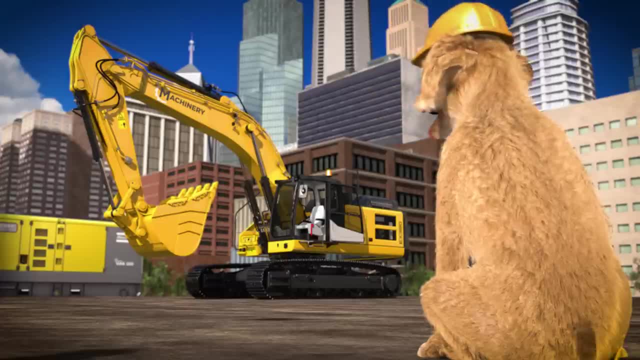 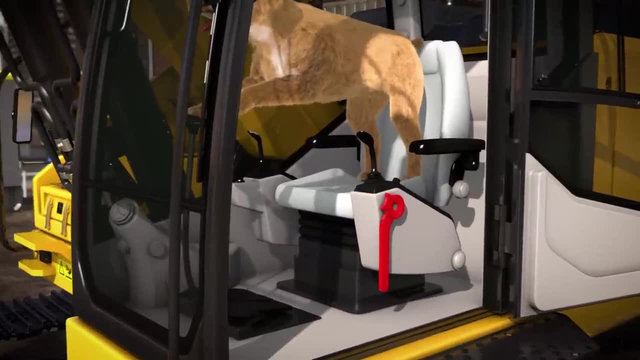 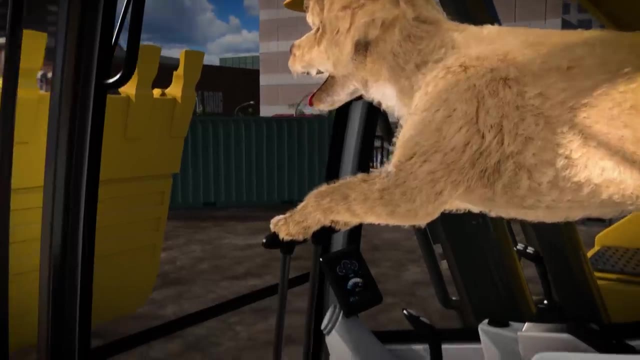 OK, let's join Lizzy in the cab and see how she controls all the different parts. Before we get started, we have to unlock the safety lock lever so Lizzy can use the controls. These handles are used to drive each track To move forward. 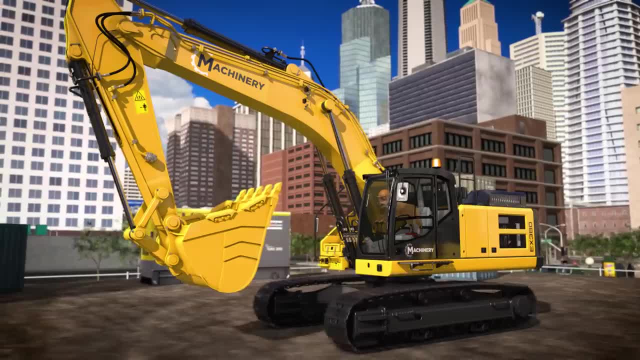 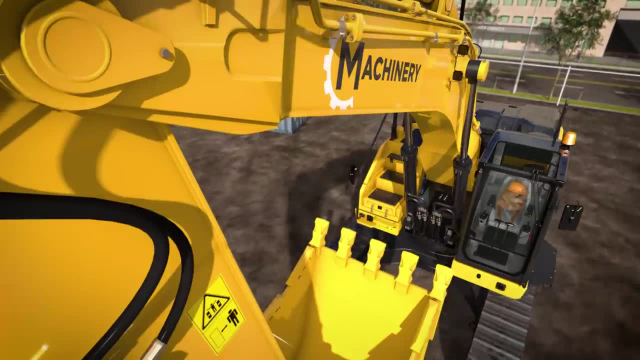 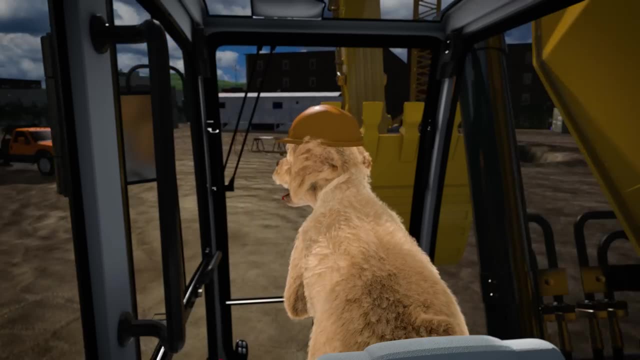 Lizzy will push both of the handles forward To move backward. Lizzy will pull the handles back To turn the whole excavator. we can make one track go backward and one track go forward like this, But we don't always have to use the tracks. 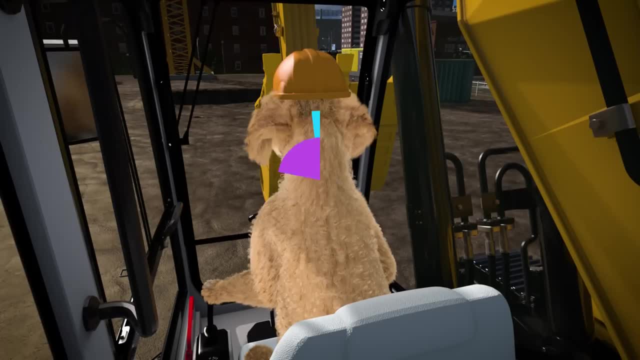 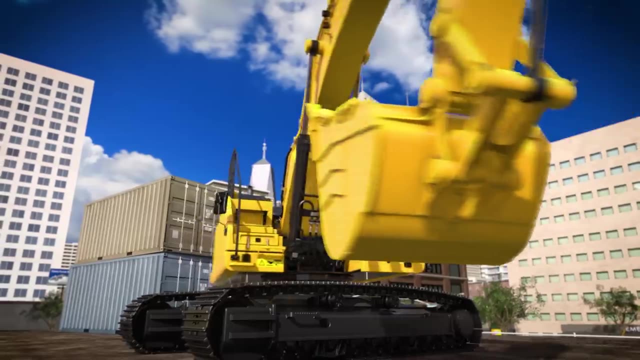 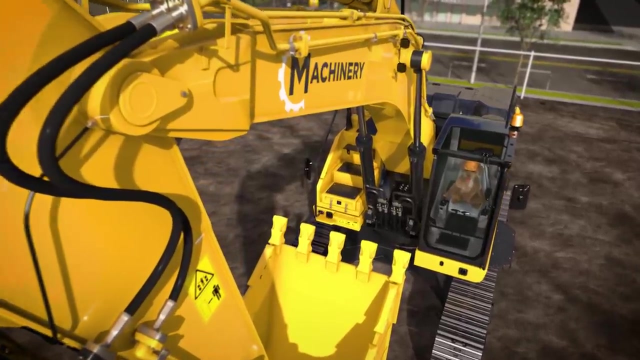 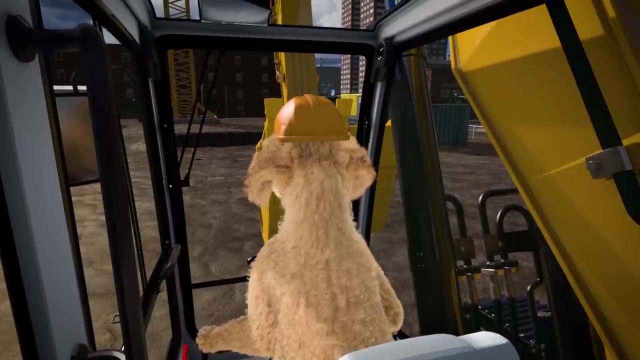 to turn the excavator. We can also swing just the house by pushing the left joystick to the sides like this. Now for the really fun part. We can use the other joystick movements to control the big, powerful excavator arm To move the boom up. 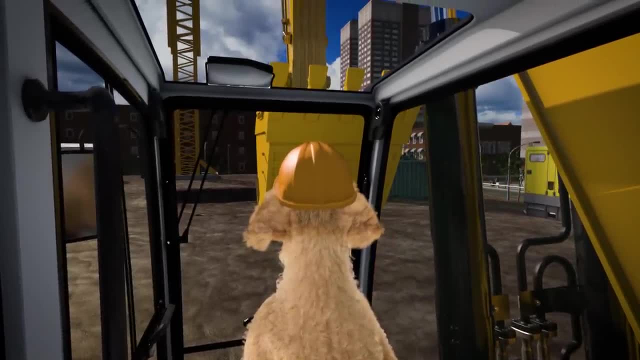 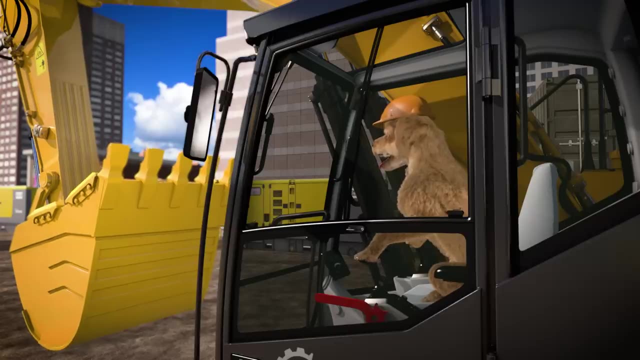 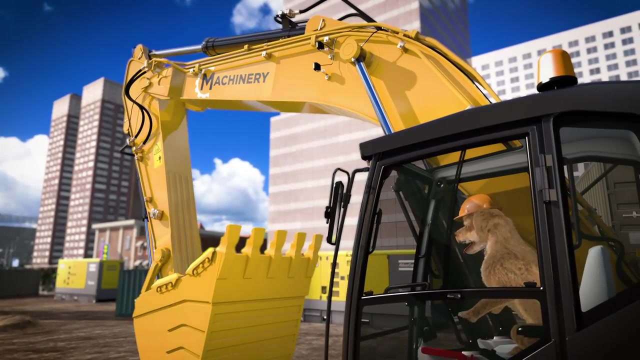 we'll pull the right joystick backward To lower the boom. we'll push the joystick forward To extend the stick. we'll push the left joystick forward like this To retract the stick. we'll pull the left joystick backward Finally to dump the bucket. 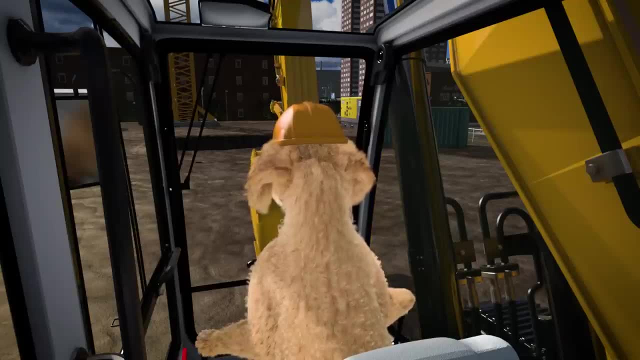 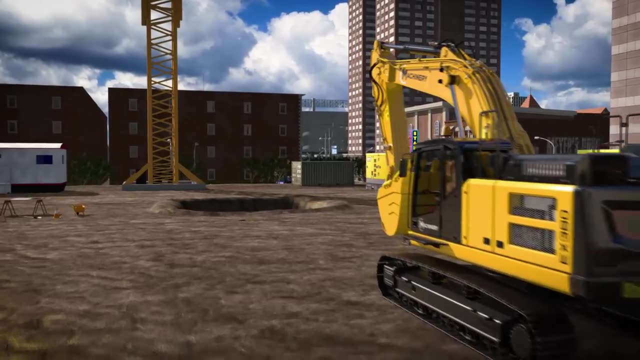 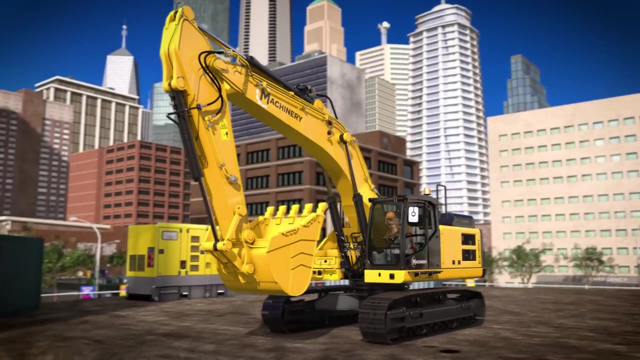 we'll push the right joystick to the right To curl the bucket in. we'll push the right joystick to the left. Awesome, Now we know the main controls of the excavator. Alright, Let's use our new skills to take out those heavy rocks. 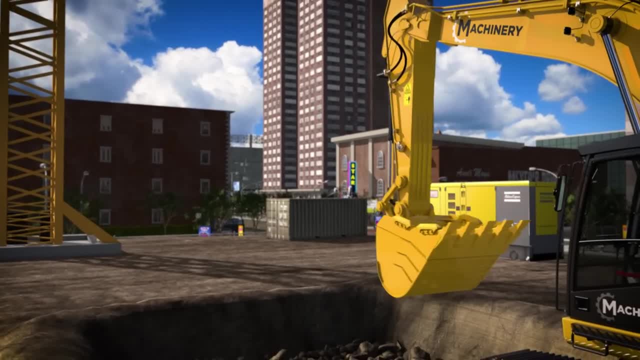 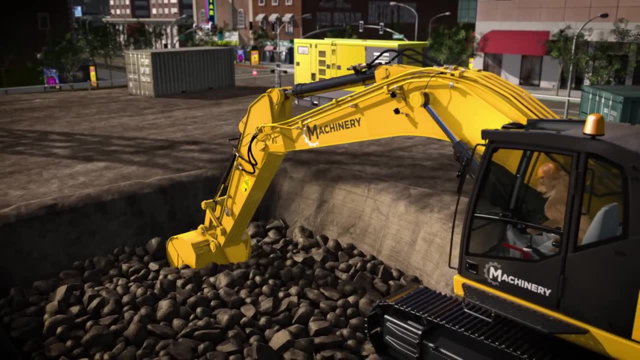 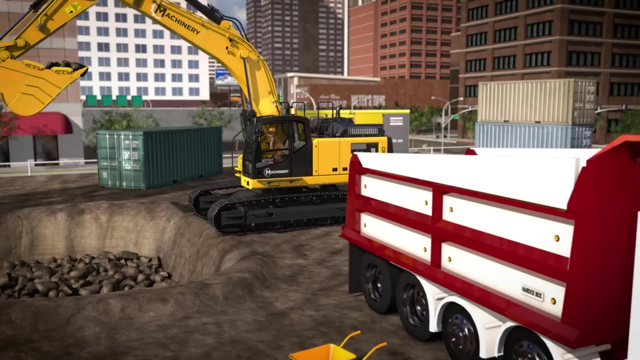 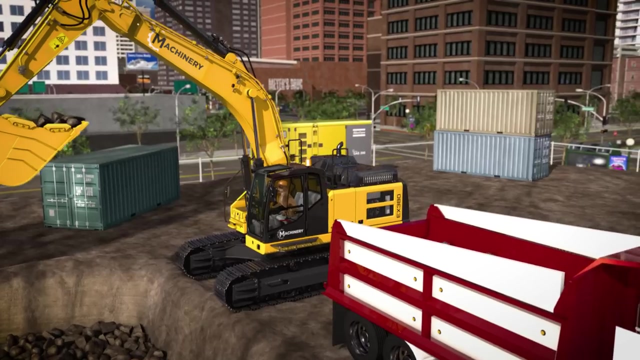 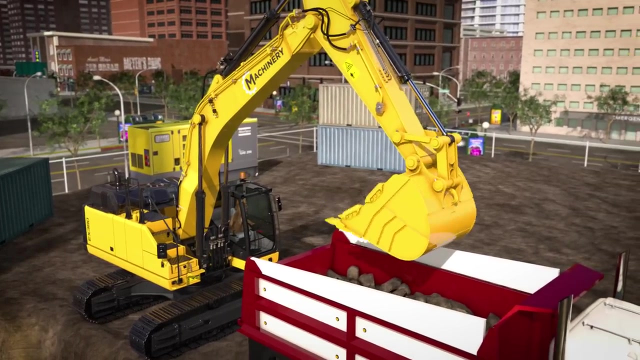 from the hole in the construction site. Whoa, it's so powerful It has no problem picking up all those heavy rocks. Hey, here comes the dump truck to take away the rocks. Let's dump them into the dump box. Nice work, Lizzy. 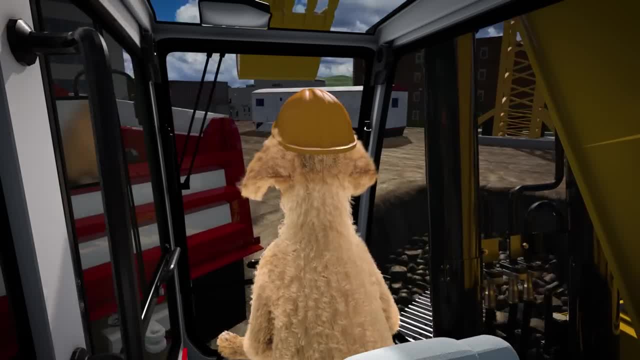 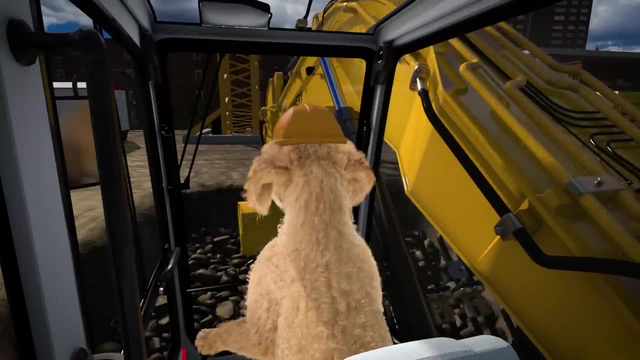 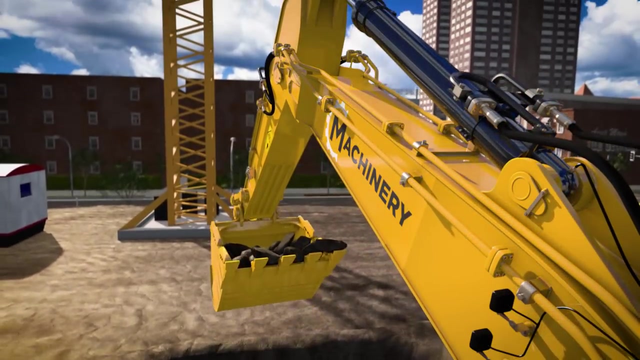 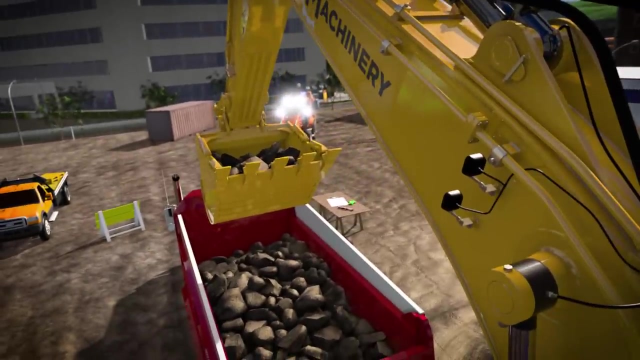 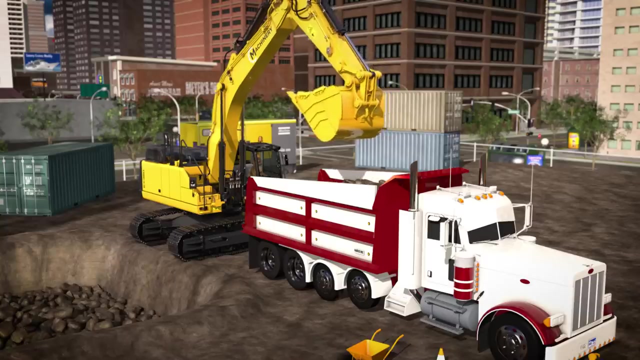 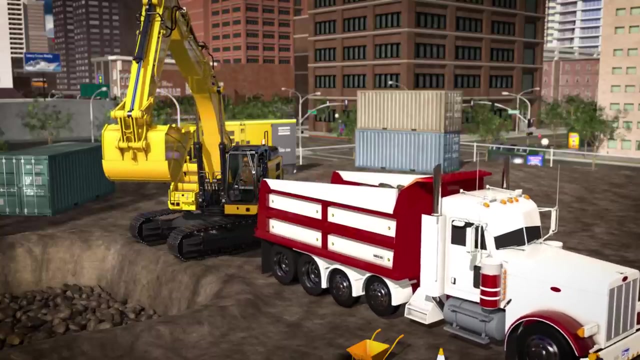 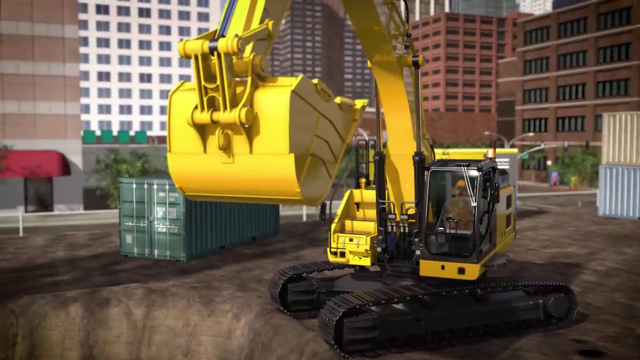 Let's get another load. Great job. Now the dump truck can take all of those rocks away. Thanks, truck driver. Wow, that was a fun day at the construction site. We learned so much about excavators and hydraulics. What do you want to learn about next? 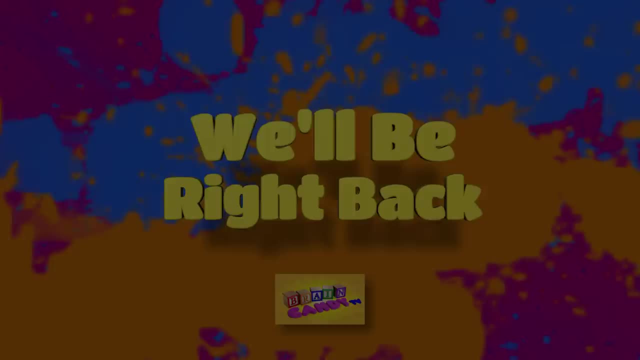 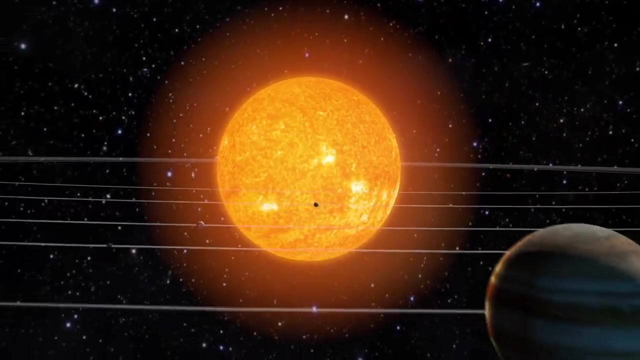 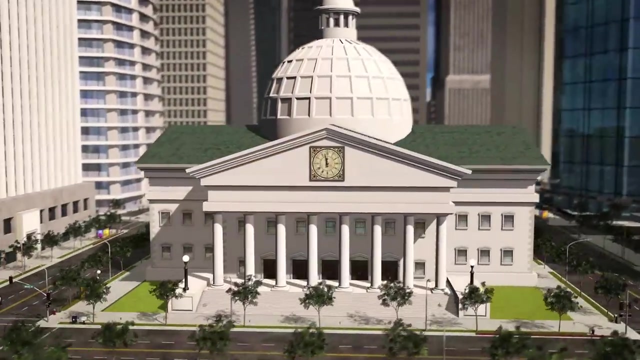 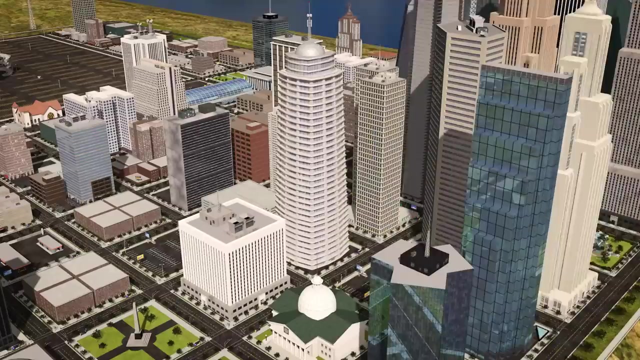 Stay tuned. we'll be back after these messages. In our previous episode, we learned all about the planets in our solar system, But do you know how far away they are from us? It's easy for us to imagine medium-sized distances and things like buildings, city blocks and even entire cities. 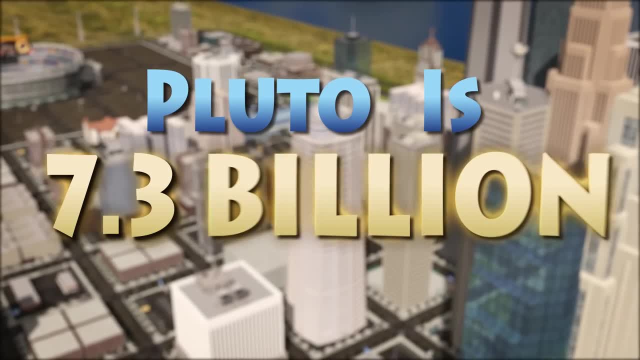 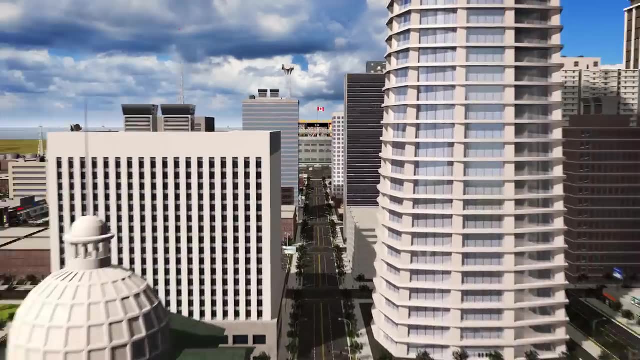 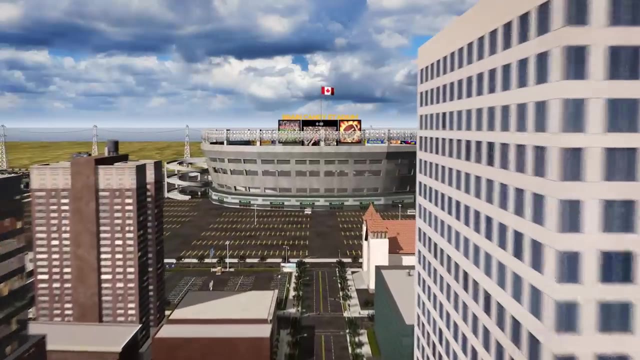 But when someone says that Pluto is 7.3 billion kilometers away, what does that really look like? For an easier way to picture how gigantic our solar system is, let's build a scale model of our solar system in a city and see how far away the planets really are. 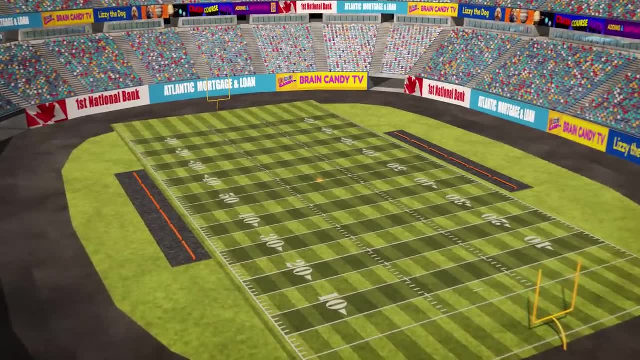 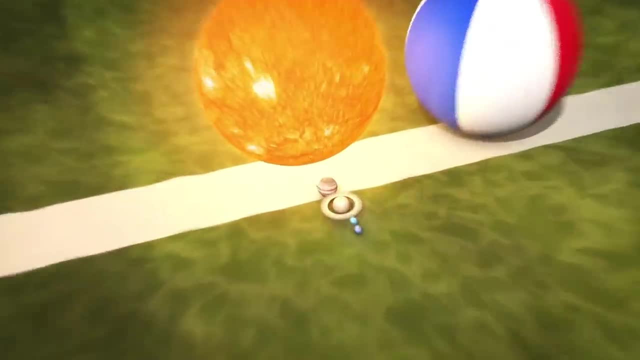 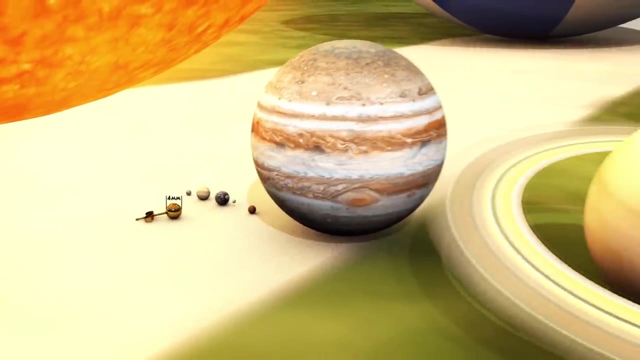 We'll start in an American football field with the sun placed at the 50-yard line and shrunk down to the size of a 44-centimeter beach ball. At this scale, Earth and Venus are the size of a solar system. Earth is a small stud earring only 4 millimeters in diameter. 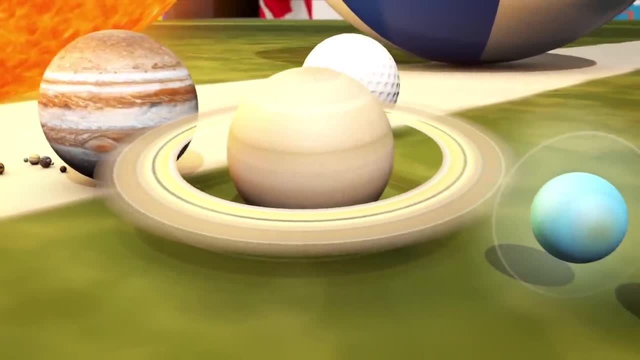 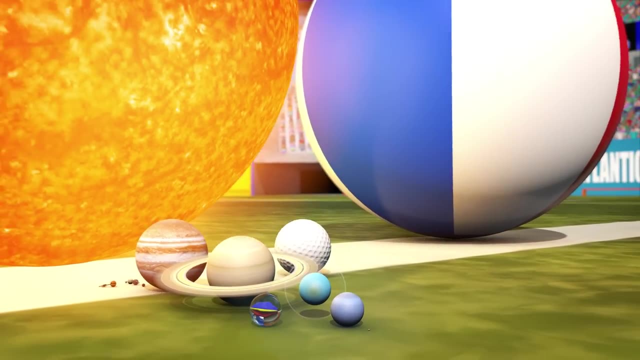 Jupiter is around the size of a golf ball, Uranus and Neptune are the size of a small marble, And our Moon and Pluto are closer to the size of a round candy sprinkle, only 1 millimeter wide. Now let's move them to their proper place. 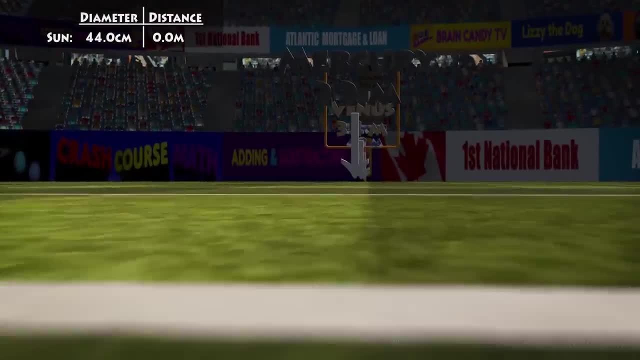 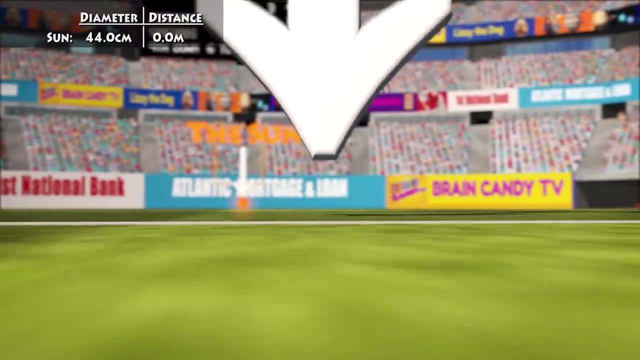 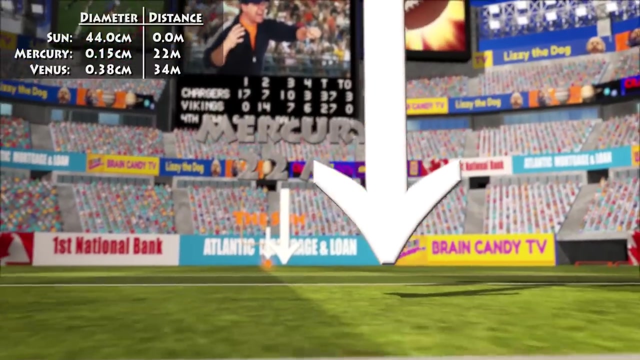 based on their farthest distances from the sun, We'll find Mercury near the 26-yard line, or 22 meters from the sun. That's equal to nearly 70 million kilometers at actual scale. Venus will be near the 12-yard line 34 meters from the sun. 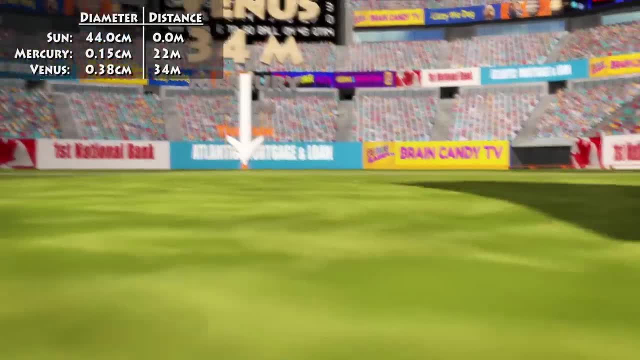 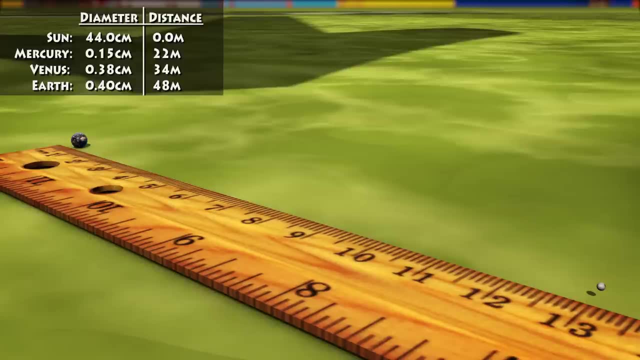 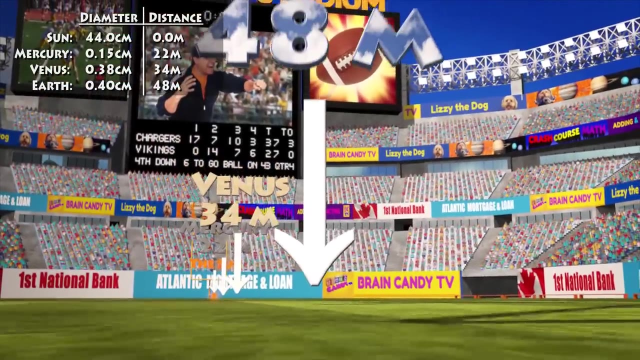 Earth can be found inside the end zone at 48 meters from our beach ball sun, And our little candy-sprinkle-sized Moon is around 13 centimeters from the earring-sized Earth. To find Mars, we'll have to get up to the middle of the lower seating section. 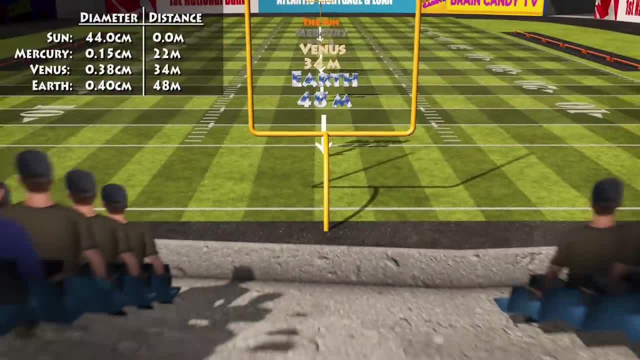 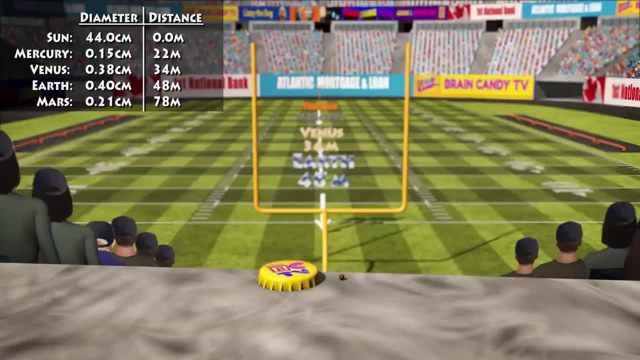 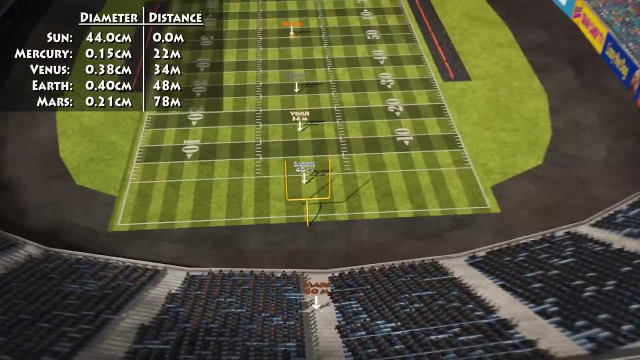 around 80 meters from the sun. At this scale, Mars is only 2 millimeters in diameter, as you can see, compared to this bottle cap After Mars, the planets are much farther apart. To get to Jupiter, we'll have to head out 260 meters. 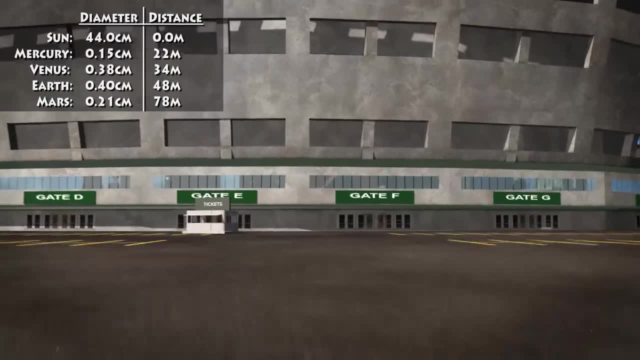 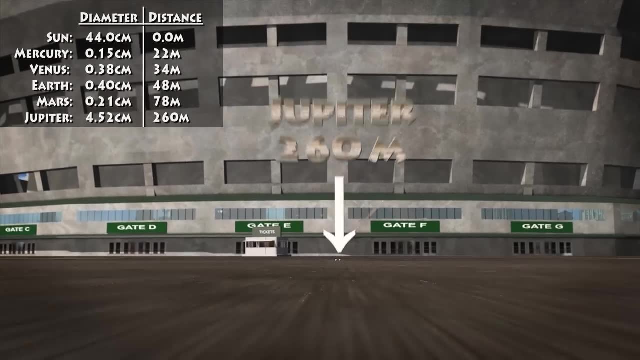 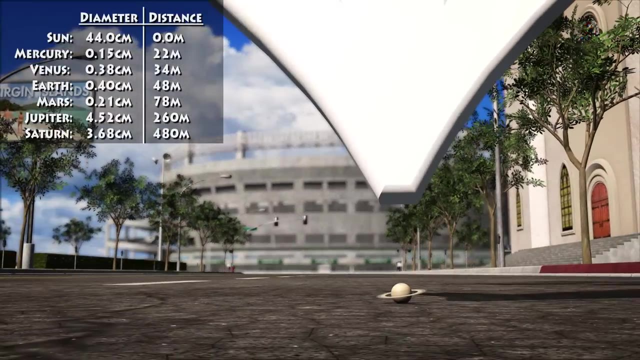 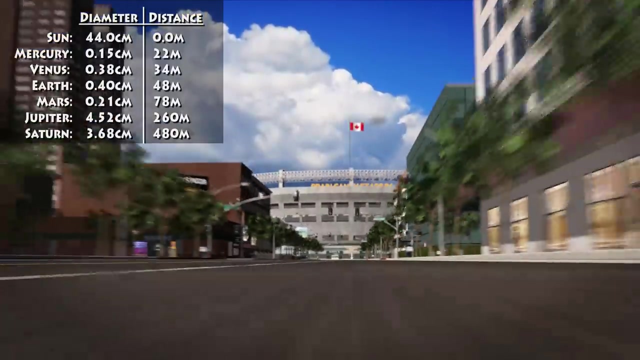 or 850 feet, which is halfway into the parking lot. Saturn will take us all the way through the parking lot and to the edge of the first block of the city, Or 480 meters from the sun. Uranus is over 5 city blocks past the parking lot. 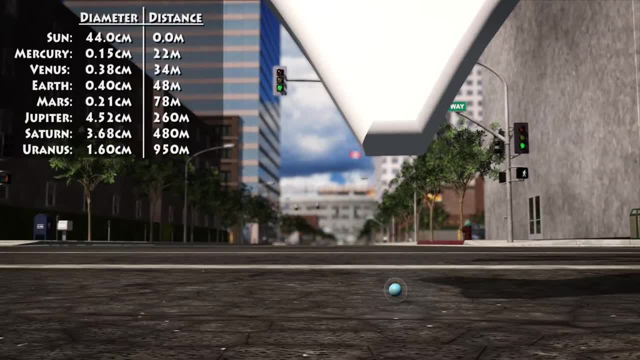 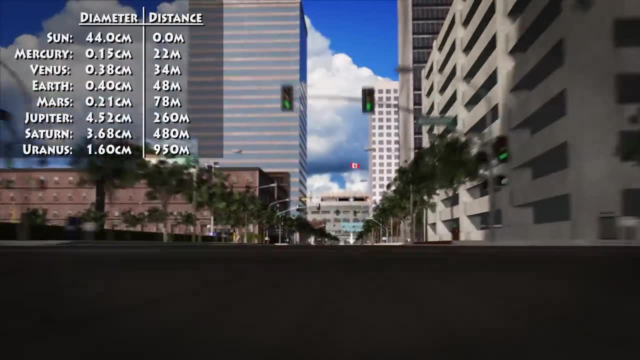 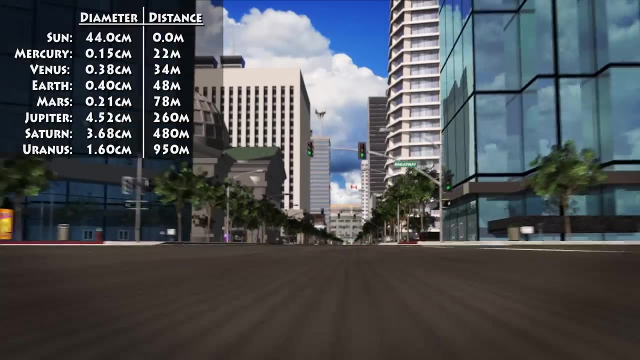 That's 950 meters from the center of the stadium. Our small marble-sized Neptune takes us right to the edge of our model city, almost 10 blocks from the parking lot and 1.43 kilometers or 0.89 miles from the sun.